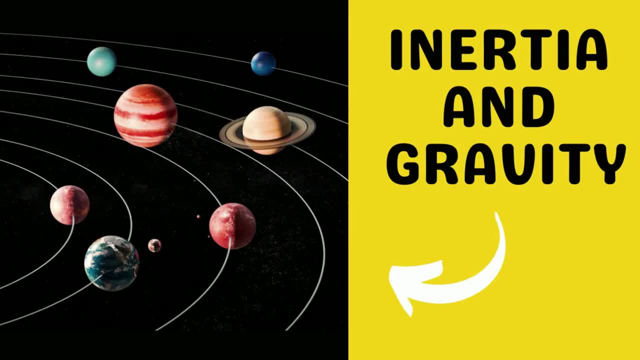 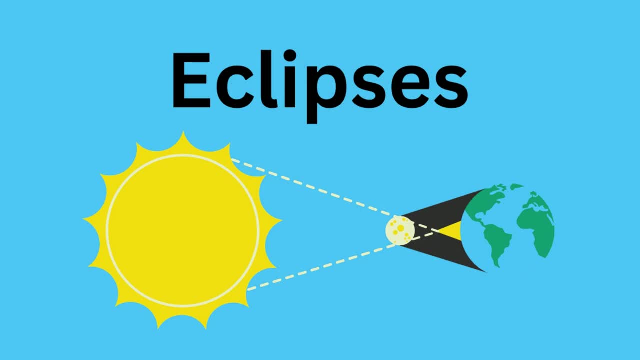 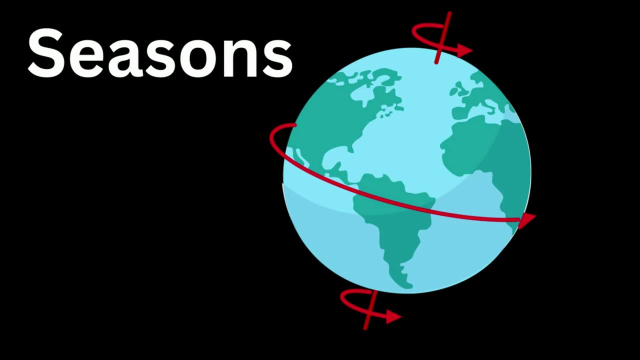 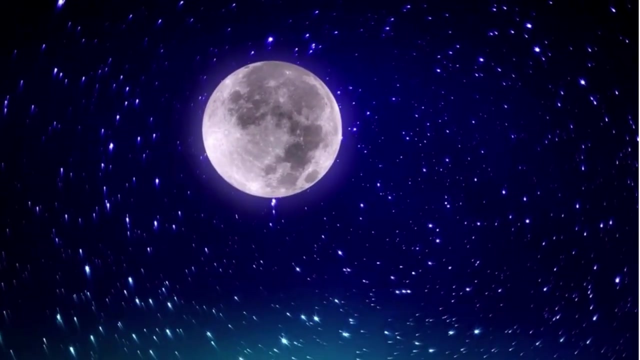 gravity and inertia working together, comets, asteroids and meteoroids, phases of the moon, types of eclipses like solar and lunar, and how the tilt of the Earth impacts seasons. So let's get started. From the perspective of the stars moving, it is very easy to assume that the Earth is at the center of the universe. 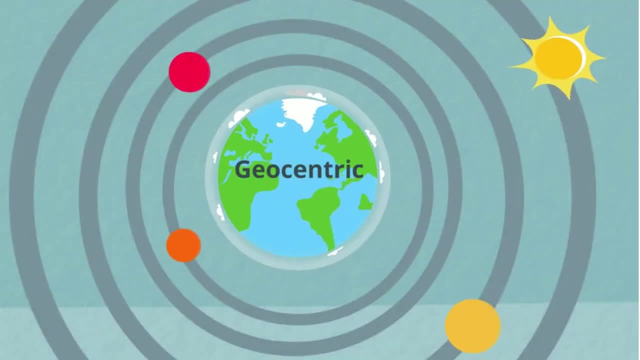 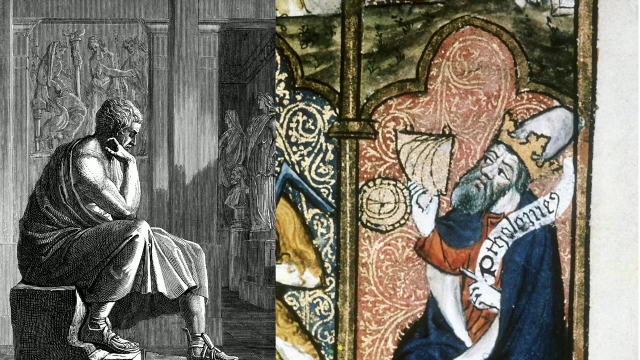 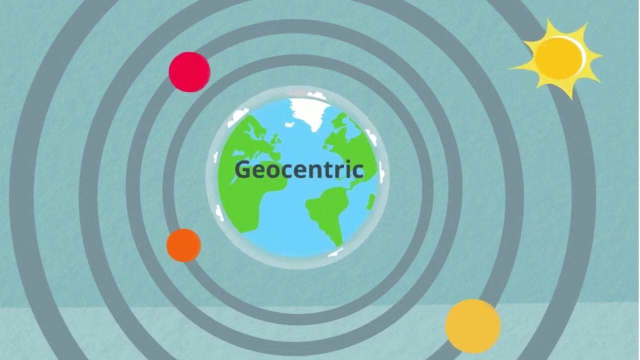 This was the accepted theory, called the geocentric model. for many years, Great minds like Aristotle and Ptolemy proposed and supported this view of the universe. Geocentric means Earth-centered, And it just seemed right. However, there were some problems. For example, sometimes the planets appear to be going backwards or to have a retrograde motion. 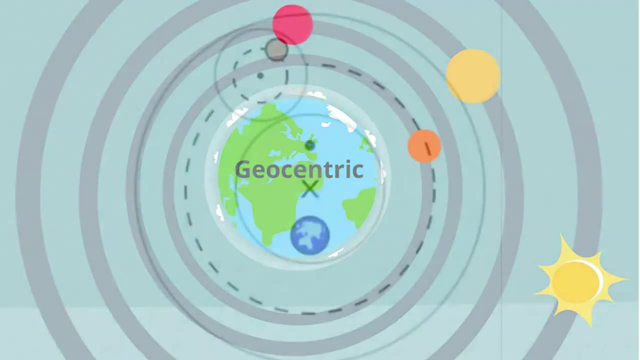 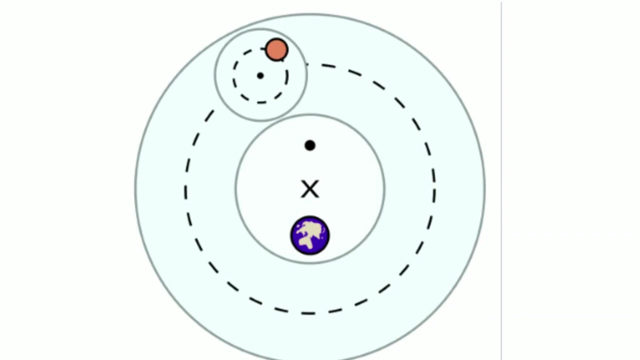 In order to explain this, small orbits called epicycles, which are orbits inside the orbit, were proposed to help explain this backwards motion. This model of the Earth being the center did not sit well with Copernicus and in 1543 he proposed: 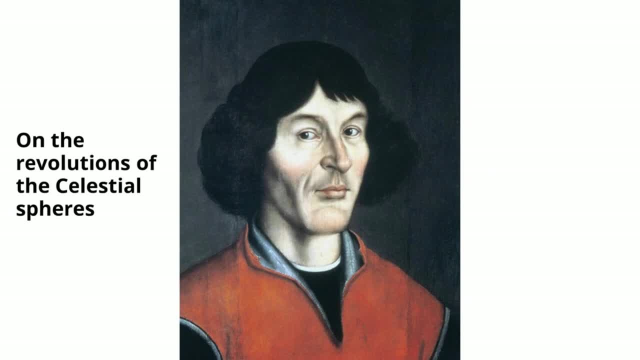 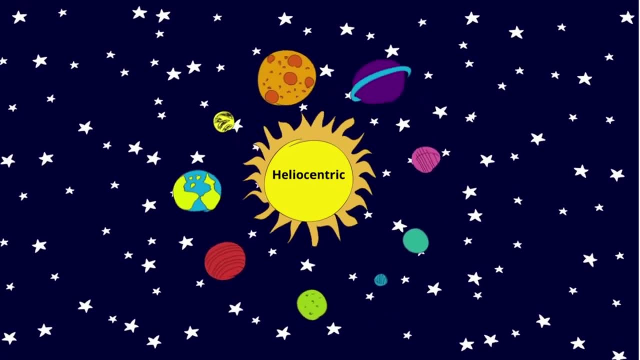 On the Revolutions of the Celestial Spheres, in which he explained what many had suspected: that the Sun is at the center of the universe and that we move on Earth along with the other planets around the Sun. This is called the heliocentric model. 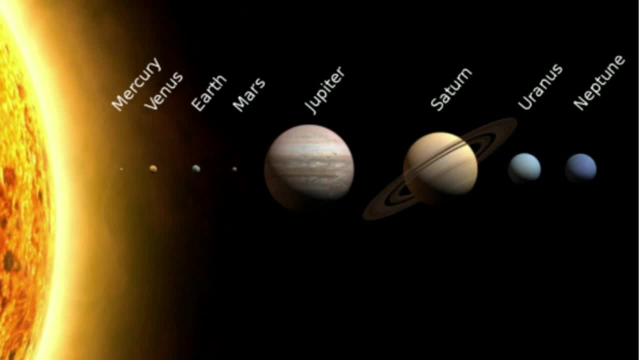 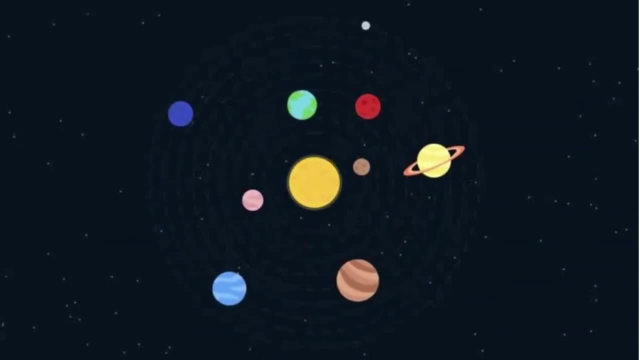 He proposed that each orbit was a circle and the Earth, like other planets, revolved around the Sun. This solved several problems, including the retrograde motion of the planets, arguing that such motion was only perceived or apparent, rather than real, With the help of his technology. 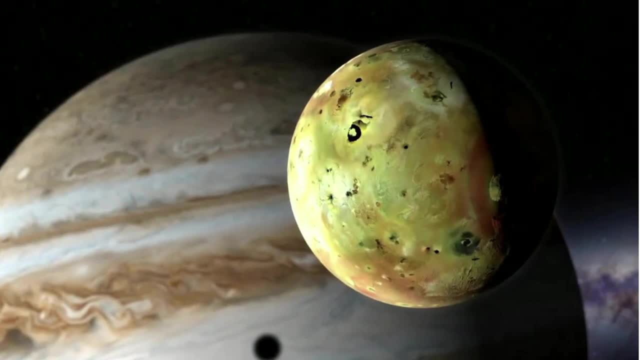 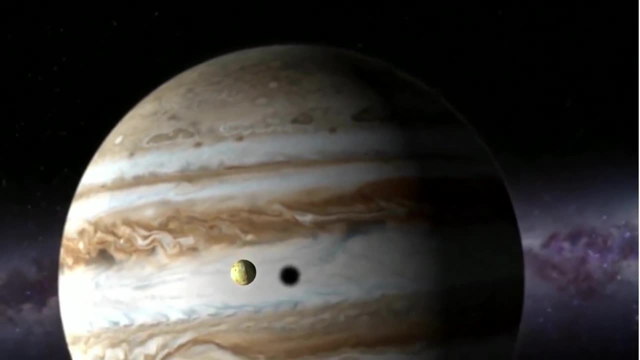 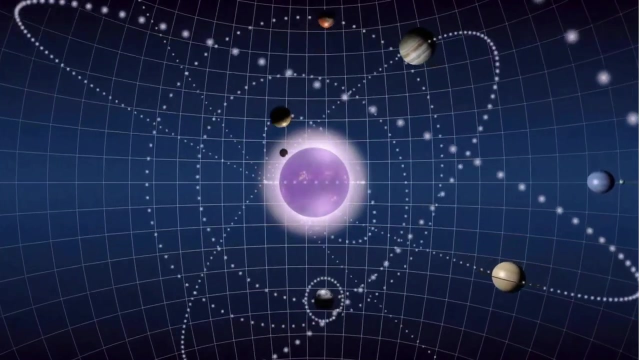 With the help of his technology, the telescope Galileo-Galilei discovered the moons of Jupiter and observed that small objects revolved around larger ones. Johannes Kepler proposed that the orbits of the planets were not perfect circles but ellipses. Our planets travel in an ellipse and actually speed up when closer to the Sun and slow down when further away. 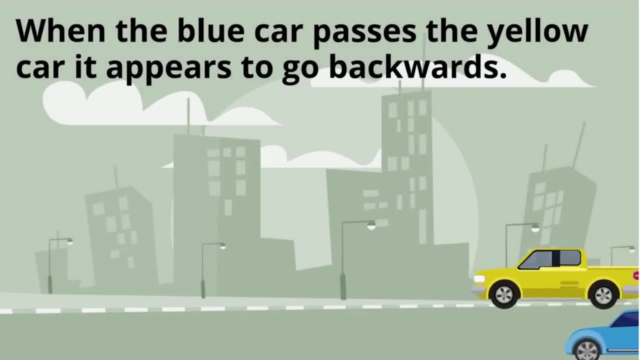 The retrograde motion of the planets was explained because it is caused by the planets that move more quickly past other planets. and it appears that the planets move more quickly past other planets. Sir Isaac Newton proposed his laws of motion to help explain how objects interact with the world and each other. 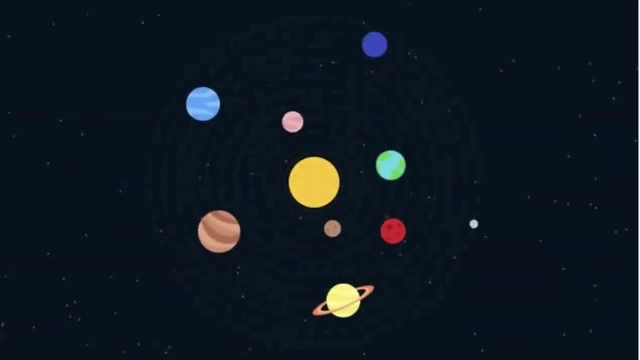 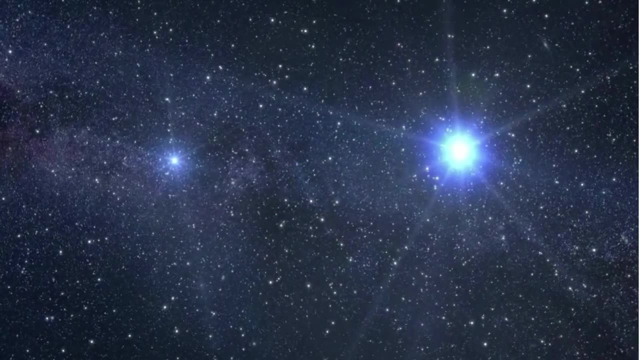 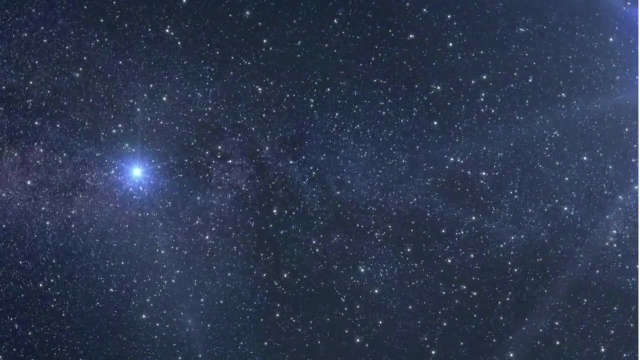 and its laws of gravity identified the responsible force behind celestial motion. We now know that the Sun is one of many stars and is not the actual center of the universe, but the planets do revolve around the Sun and not the other way around. Let's take a look at what makes up a solar system. 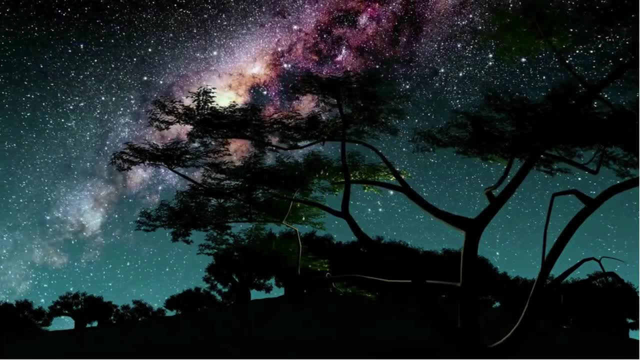 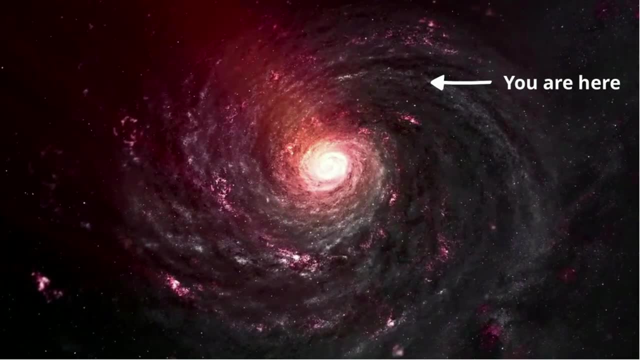 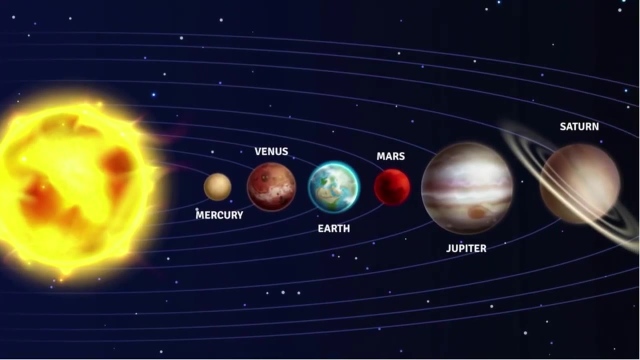 a galaxy and a universe. Our solar system is located in the Orion arm of the Milky Way galaxy. It consists of the sun and the objects that orbit it either directly or indirectly. This includes several objects. First, the planets. The eight planets in order from the sun are: 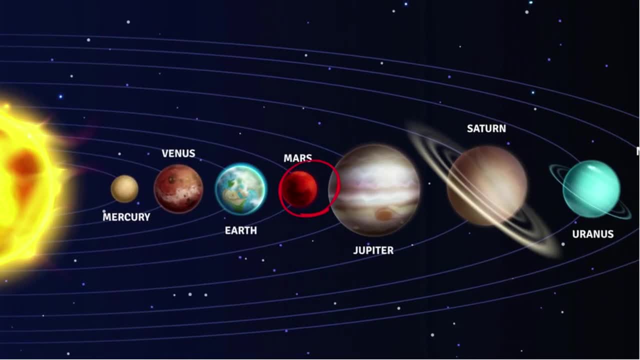 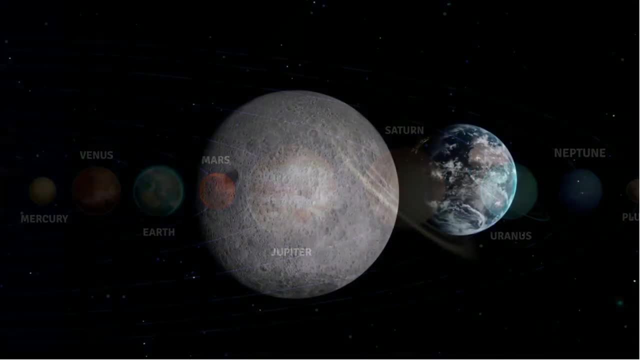 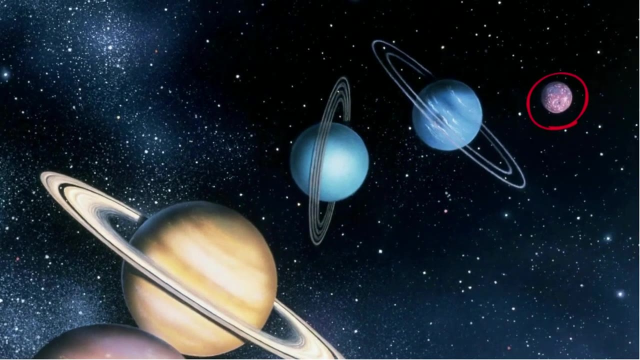 Mercury, Venus, Earth, Mars, Jupiter, Saturn, Uranus and Neptune. Indirect objects include the moons that revolve around the planets. There are over 200 moons in our solar system. In addition, you have dwarf planets like Pluto and small solar system bodies which are comets. 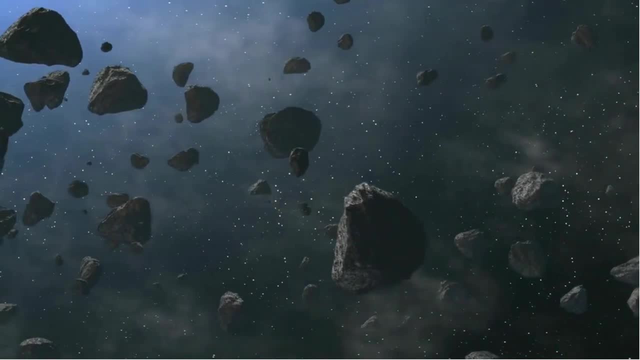 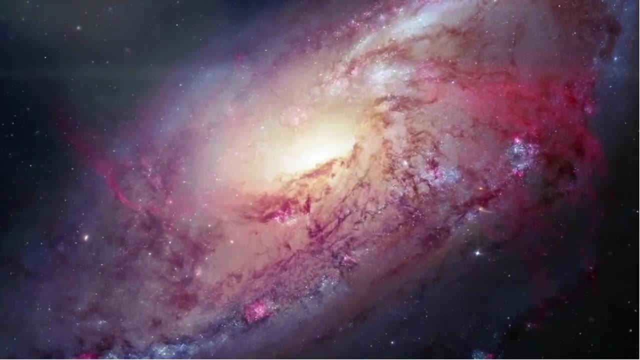 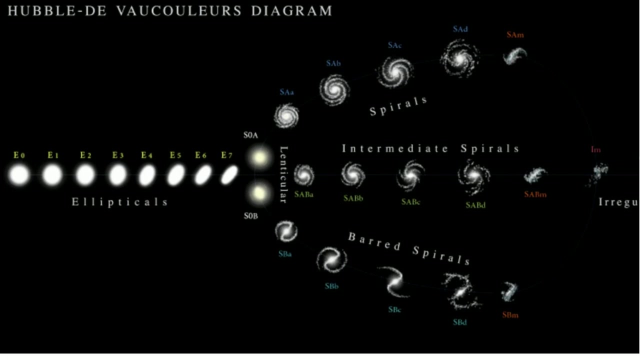 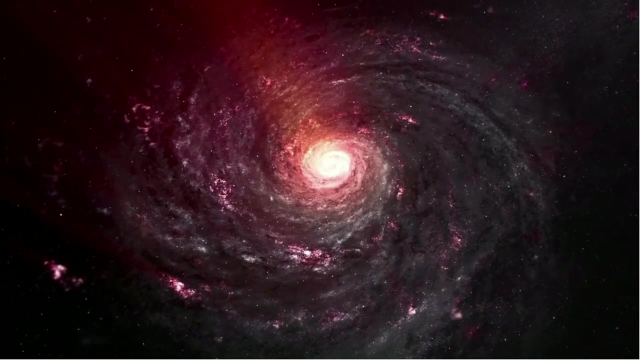 asteroids, trans-Neptunian objects. A galaxy is larger than a solar system and it is a gravitational bound collection of stars, along with their planets, gas, dust and dark matter. There are at least three main types of galaxies: Electrical, spiral and irregular. Galaxies are huge and range in size from dwarfs with just a. 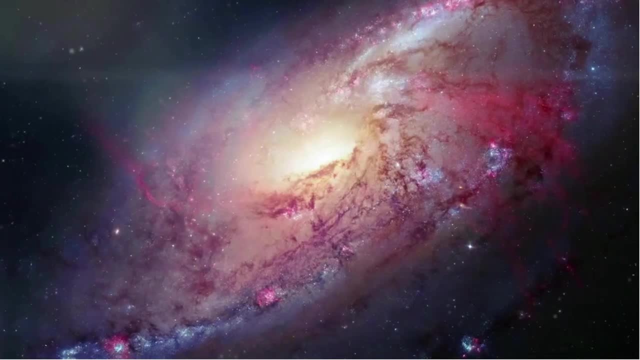 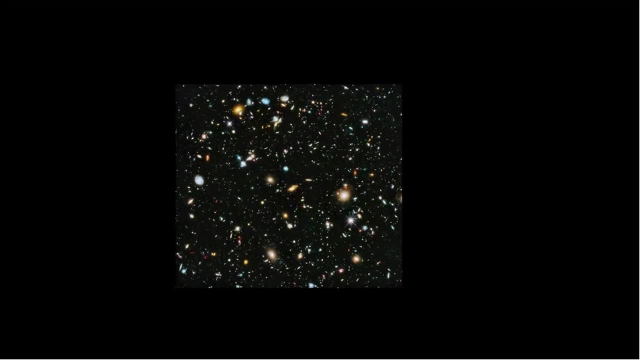 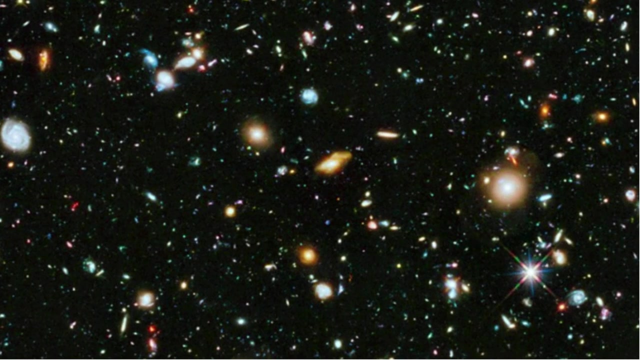 few hundred million stars to giants with 100 trillion stars each orbiting its galaxy's center of mass. It is estimated that there are over 1 billion galaxies. If you take a look at this picture from the Hubble telescope, each of these small dots is a galaxy. 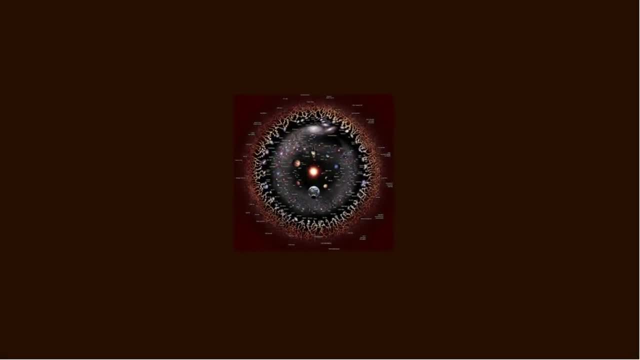 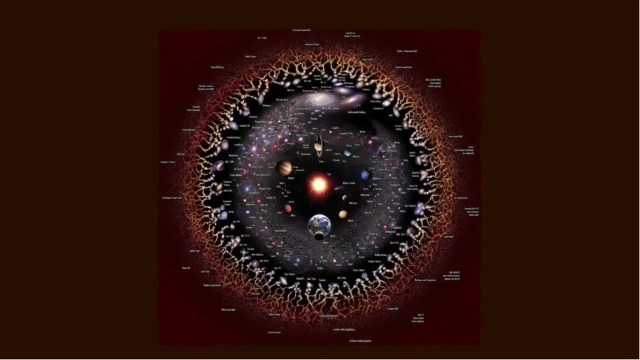 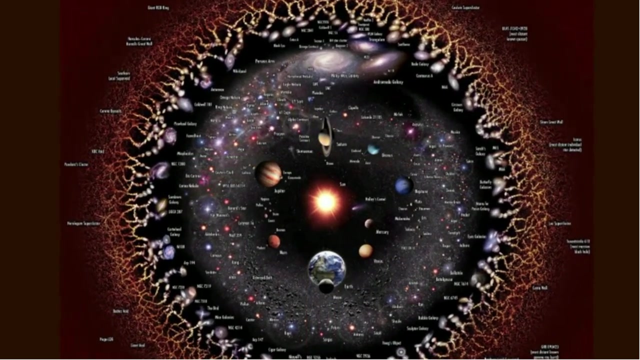 Finally, the universe. It is a vast expanse of space which contains all of everything in existence. The universe contains all the galaxies, stars and planets. The exact size of the universe is unknown. Scientists believe the universe is still expanding outward. This clip gives you a little idea of the size of our universe. 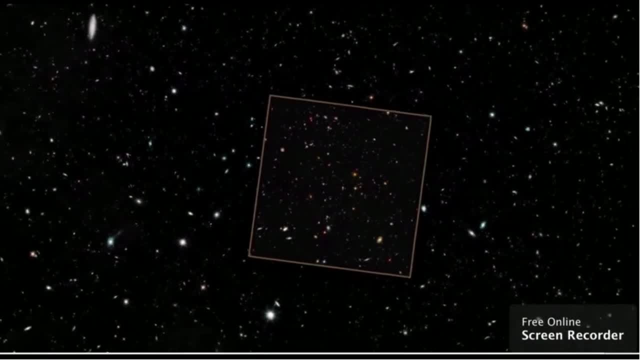 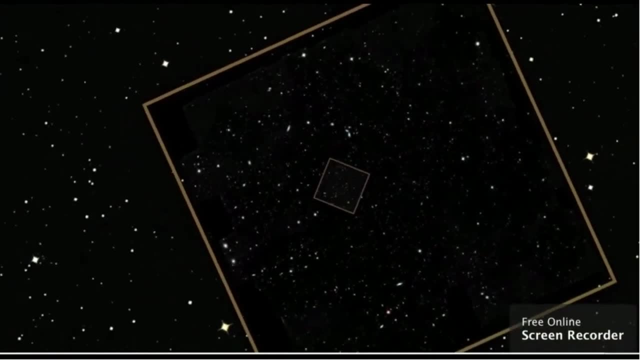 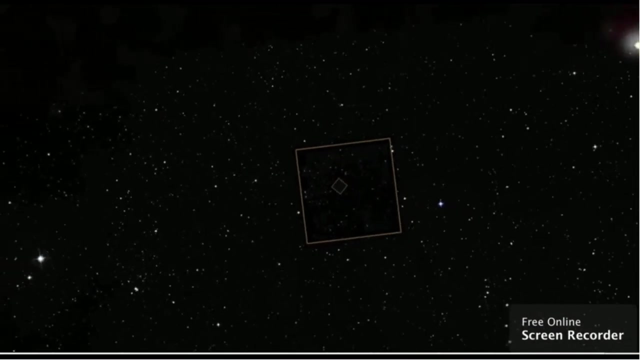 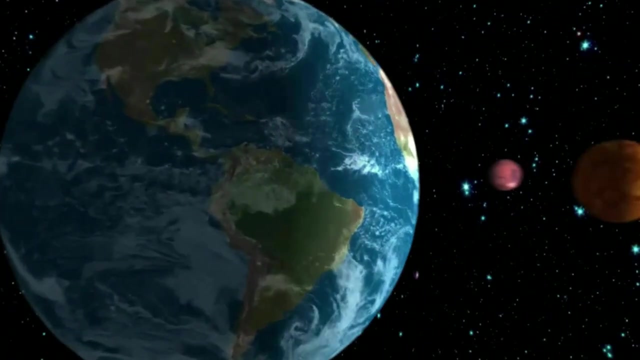 The dots that look like stars are galaxies, And galaxies contain billions of stars, And then our solar system is located around just one star. So there we go, What you will find in a solar system, a galaxy and the universe. Let's take a look at the eight planets and let's look at relative size compared to the earth. 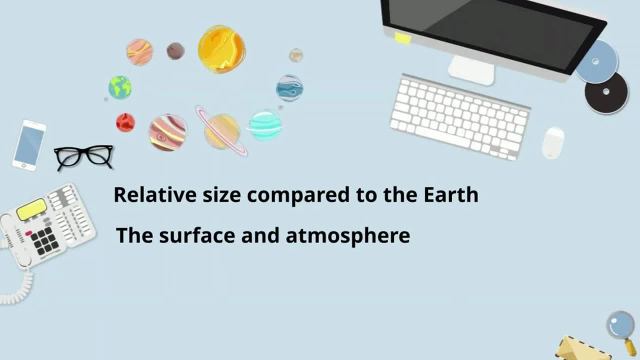 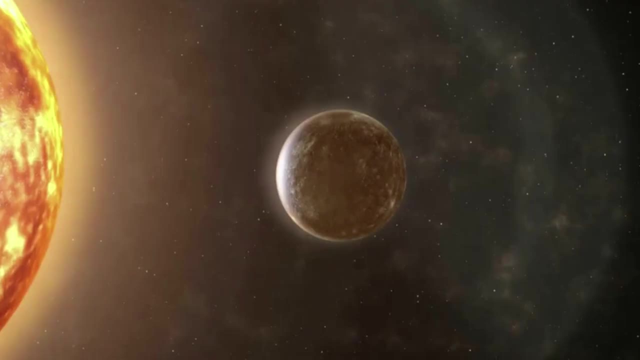 its surface and atmosphere, its relative distance from the sun compared to the earth, and its ability to support life. Up first is Mercury. Mercury is about one-third the size of the earth. It has a central core, a rocky mantle and a solid crust. 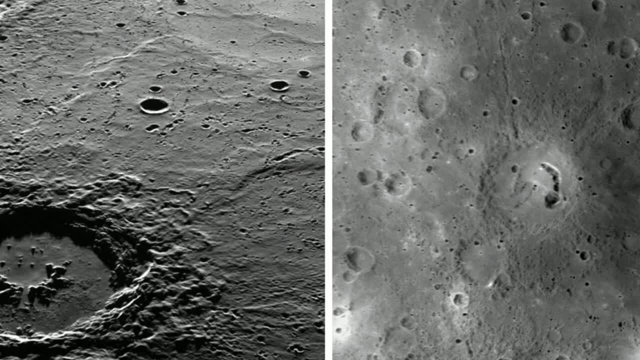 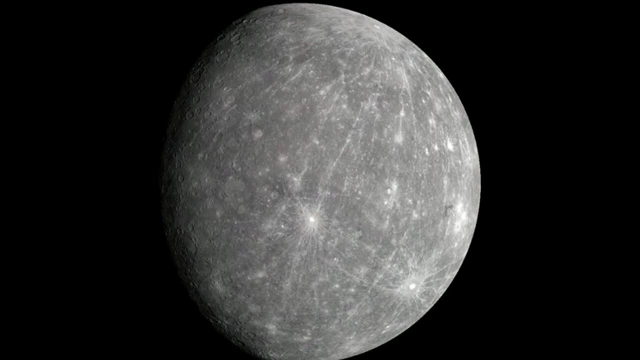 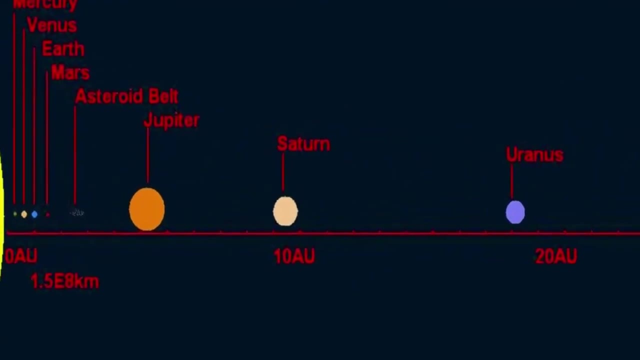 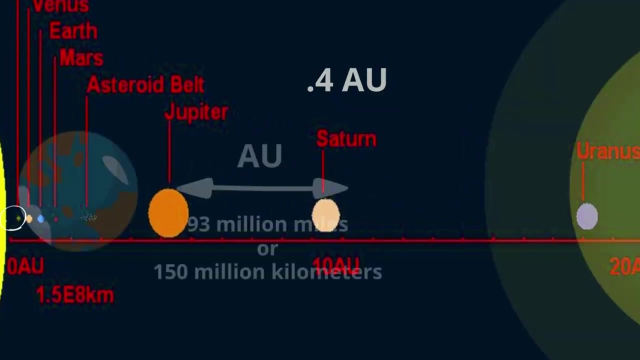 very, very thin atmosphere And is composed mainly of oxygen, sodium and hydrogen. It is point four, AU from the sun. So it's forty percent the distance from the sun than the earth is, And AU is the distance from the earth to the sun. This allows you to see if the planet is closer or further from the sun. 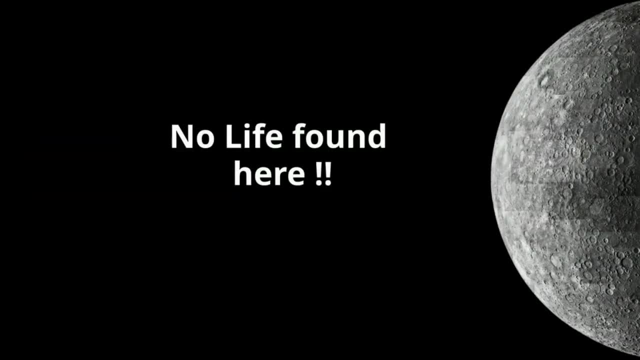 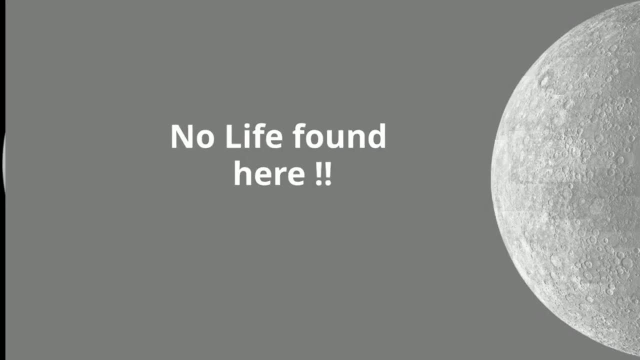 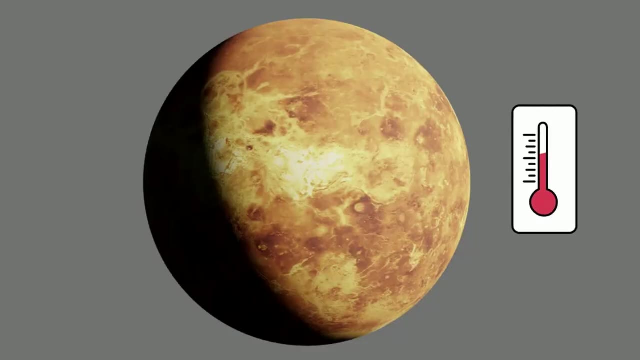 compared to the earth地 to shark. Because of the extreme temperatures and solar radiation it is very unlikely to have any life. venus is slightly smaller than the earth. it's the hottest planet in our solar system. surface temperatures on venus are around 900 degrees fahrenheit. 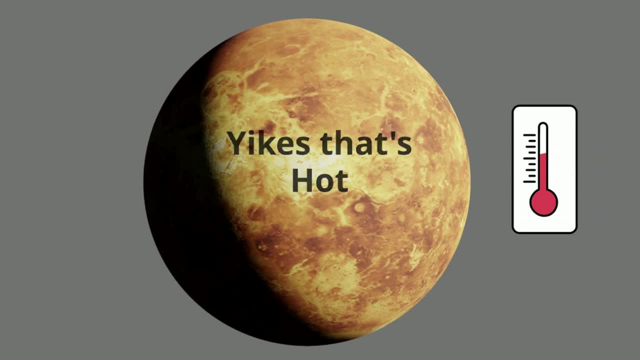 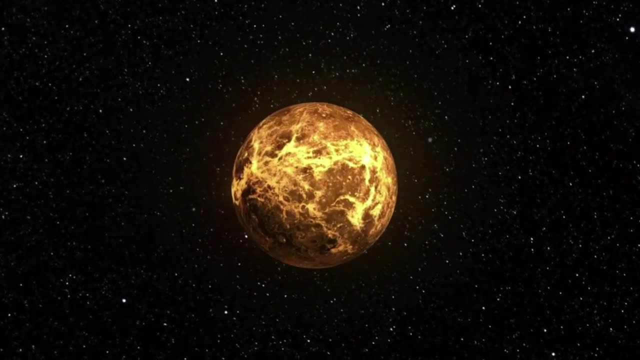 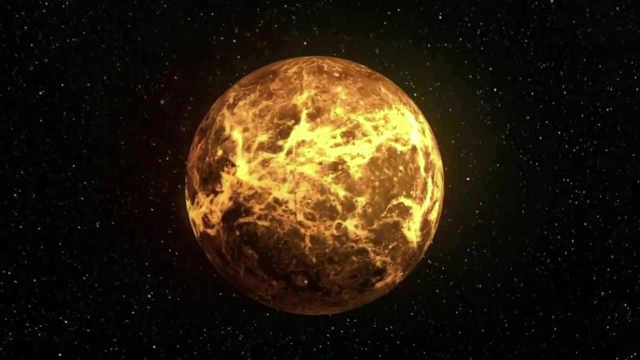 the surface is a rusty color and has mountains and thousands of large volcanoes, along with dust. the air pressure is roughly 90 times greater than the earth's due to its thick atmosphere. its atmosphere is thick and composed of 96 carbon dioxide and four percent nitrogen. the carbon 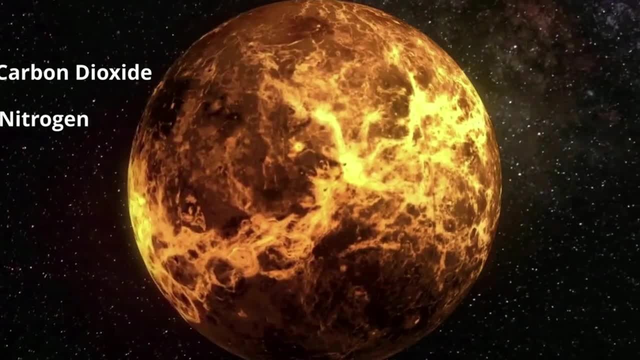 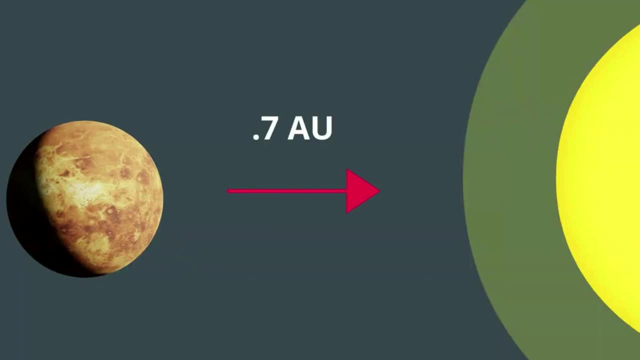 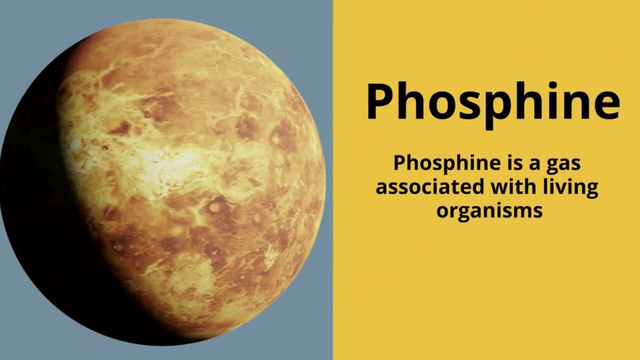 dioxide traps in heat and causes the extreme temperature. it is 0.7 au from the sun, or 70 the distance that the earth is. this is interesting. the detection of phosphine recently in the atmosphere of venus may indicate that there may be life in the atmosphere of venus for many years. 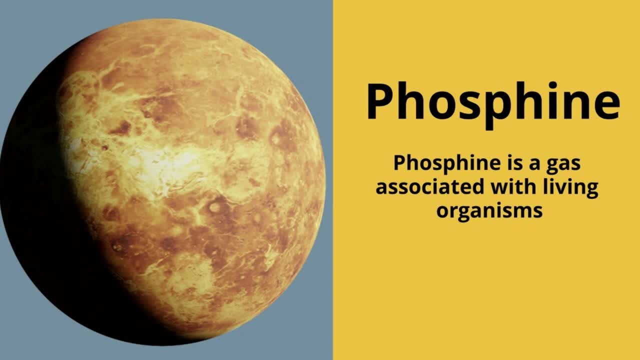 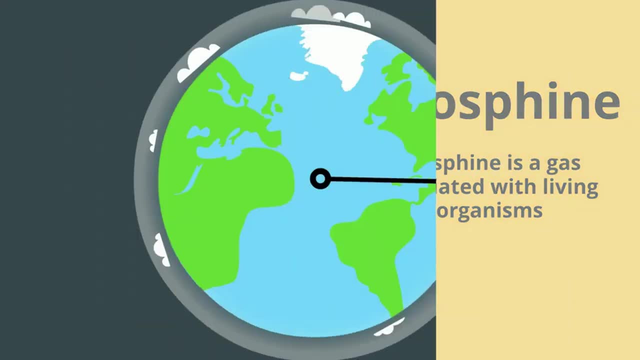 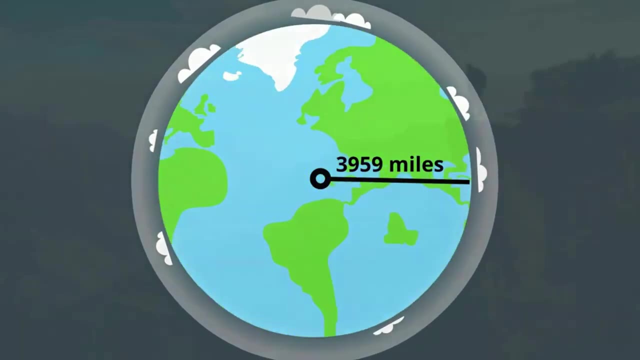 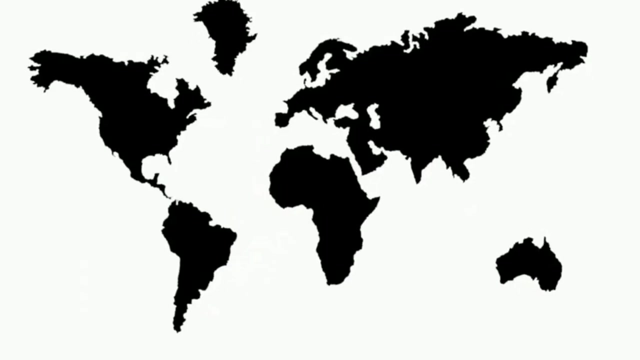 life seemed improbable on this furnace of a planet, but these recent discovery of phosphine has caused scientists to rethink. life on venus earth has a radius of 3 959 miles roughly. it has a solid surface composed of canyons, mountains, volcanoes and tectonic plates that move its atmosphere is. 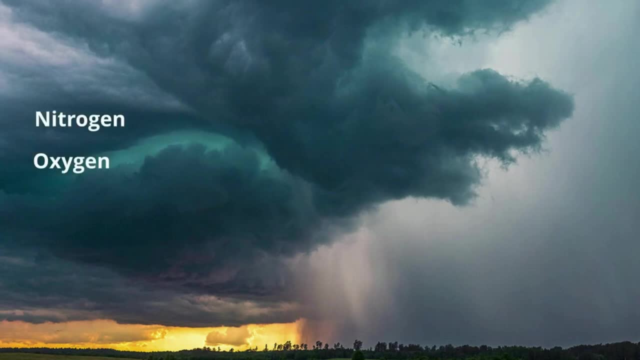 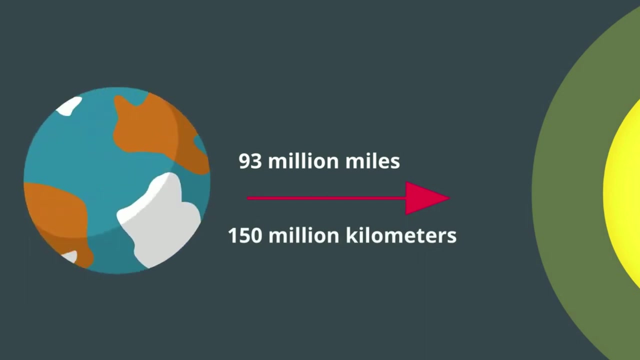 composed of 78 percent nitrogen, 21 percent oxygen, golden water and oil body flammable oceans that produce granite present in the solar system 7 cellsобщ 7 millionAND 16 million, one percent argan and less than one percent of other gas. earth is 1 au from the sun, which is roughly 93 million miles or a hundred, and 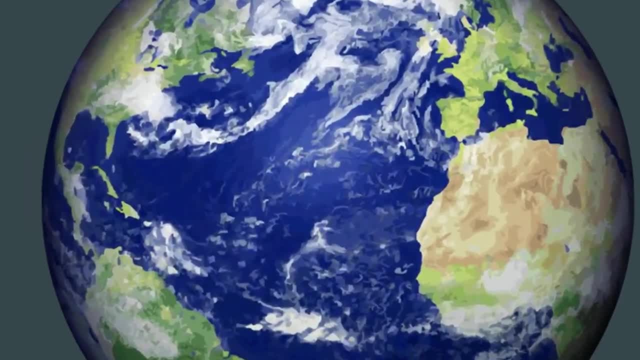 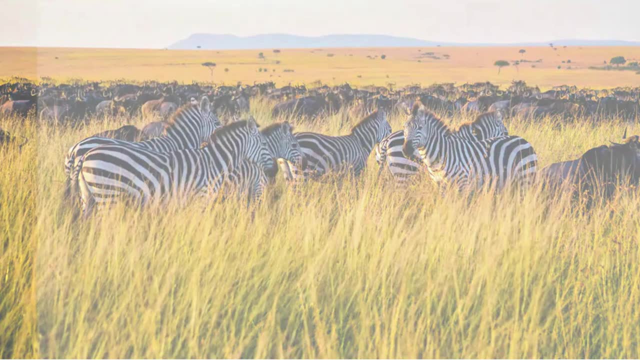 15 million kilometers on the sun. earth has a huge variety of life on it. Mars is about one-half the size of Earth. the surface of mars is covered with water. док Agっちゃ about apka. there is no energy extracted from grazio. 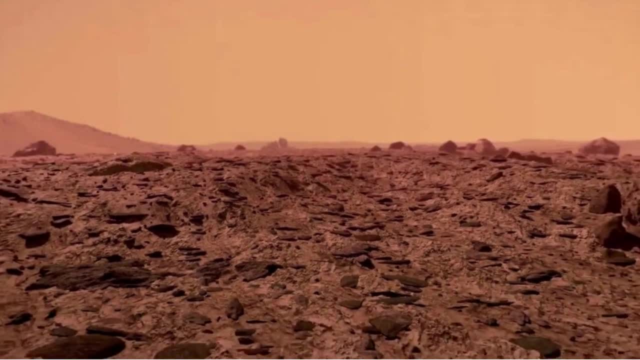 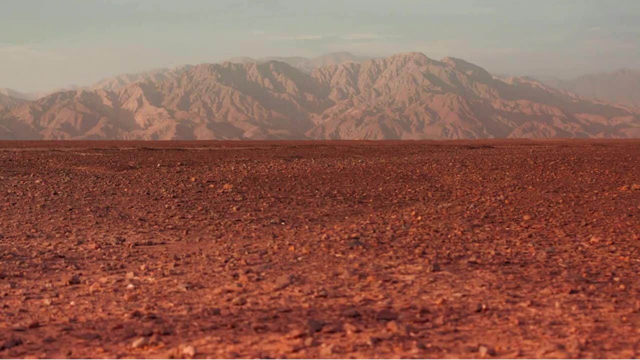 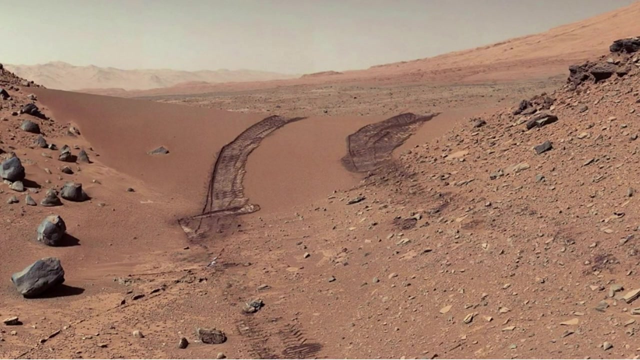 Spanish limestone and uranium beautiful destroying large ее covered with reddish dust due to the rusting of the iron in its surface. It has seasons, a huge canyon and one of the largest volcanoes in the solar system. There is a limited amount of water on Mars. 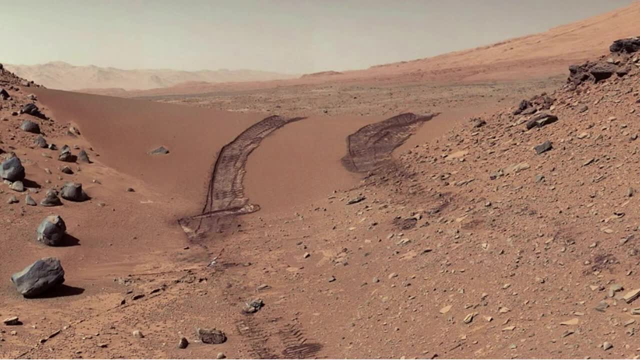 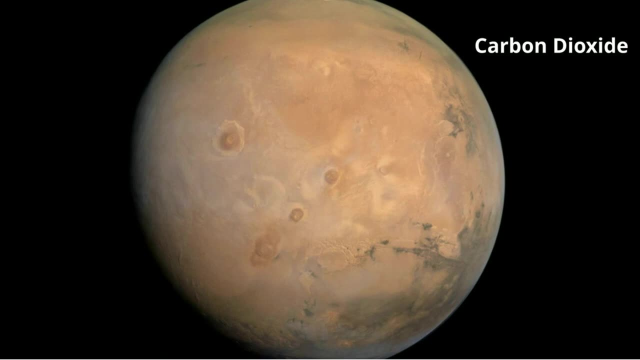 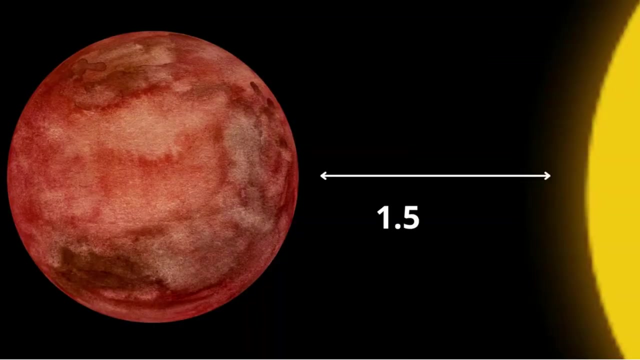 and it's found in the form of ice just under the surface in the polar regions. It has a thin atmosphere composed of 97.5% carbon dioxide, 2.7% nitrogen and 1.6% argon. Mars is 1.5 AUs from the sun. 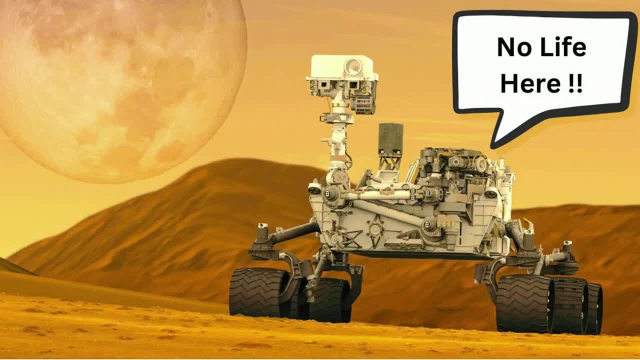 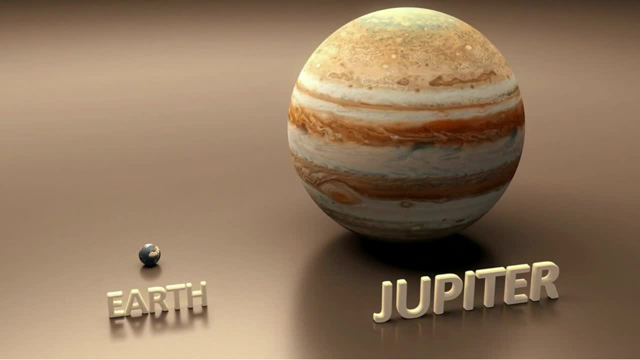 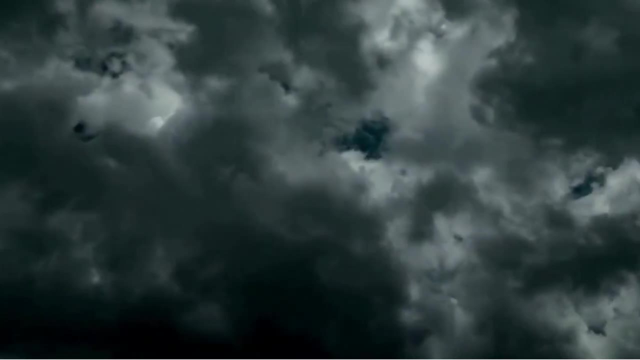 To date, no proof of past or present life has been found on Mars. Jupiter is 11 times larger than the Earth and it is the largest planet. Jupiter doesn't have a true surface. The planet is mostly swirling gases and liquids. It does have a very large ocean made of hydrogen instead of water. 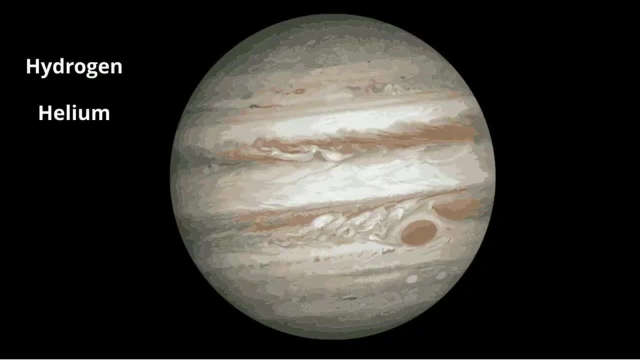 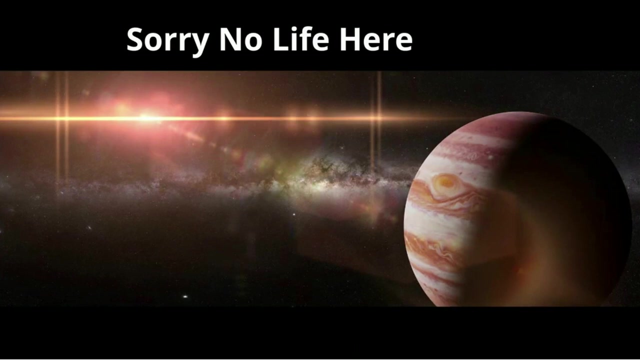 Its atmosphere is made up of 90% hydrogen and 10% helium, and it's famous for the red spot, which is a huge storm that has been raging for hundreds of years. The chances of life on Jupiter are very rare. The temperatures and pressures of this planet are most likely too extreme and vital for organisms to survive. 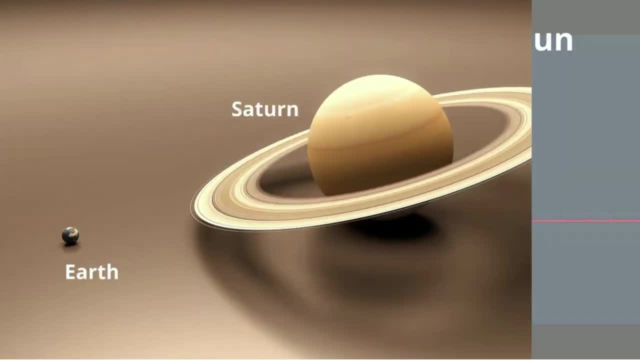 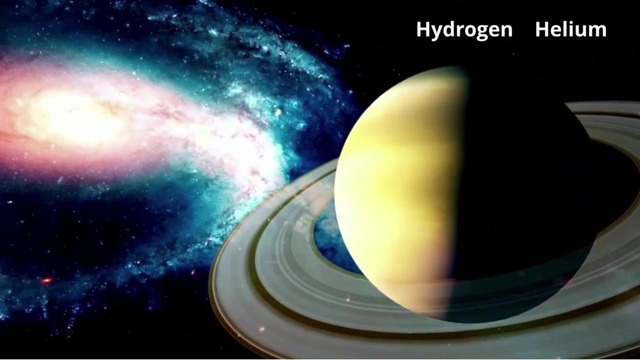 Saturn is 9 times larger than Earth. Like Jupiter, Saturn is a gas giant and therefore does not have a solid surface. Its atmosphere is similar to the sun and Jupiter, with over 95% hydrogen and 3% helium. Saturn is 9.6 AUs from the sun. 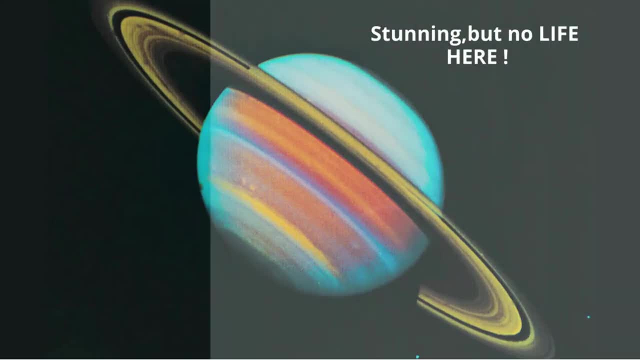 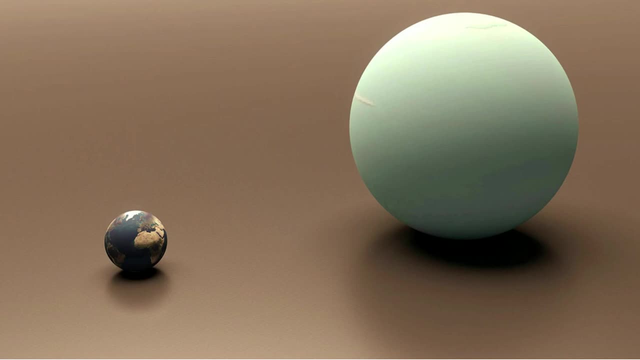 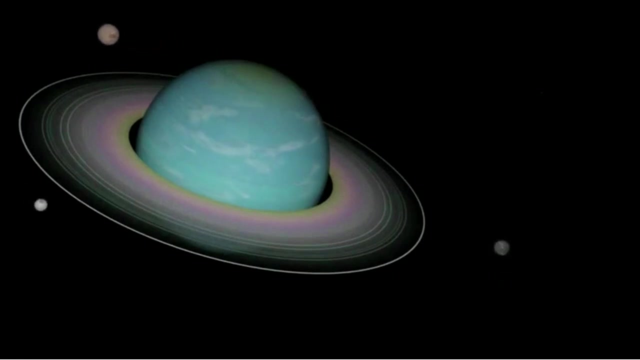 Saturn cannot support life. Uranus is roughly four times the size of the Earth. It does not have a solid surface. However, it does have very cold temperatures on its surface: minus 353 degrees Fahrenheit. It consists mainly of clouds made of ice crystals, of water, methane and some ammonia. 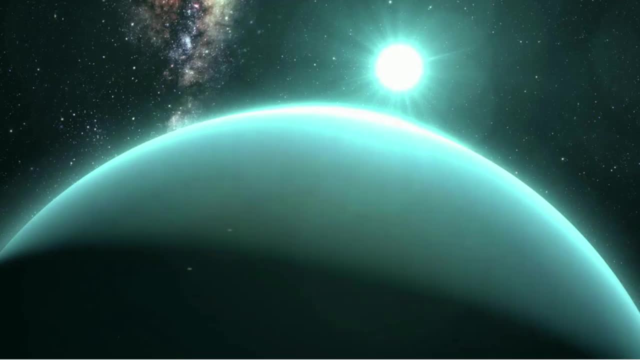 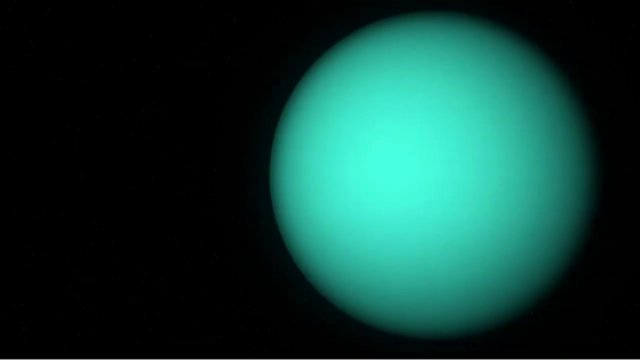 It does have a small solid core. Its atmosphere is made up roughly of 2% methane, 80% hydrogen and 15% helium. Uranus is 19.2 AUs from the sun and there is no life. 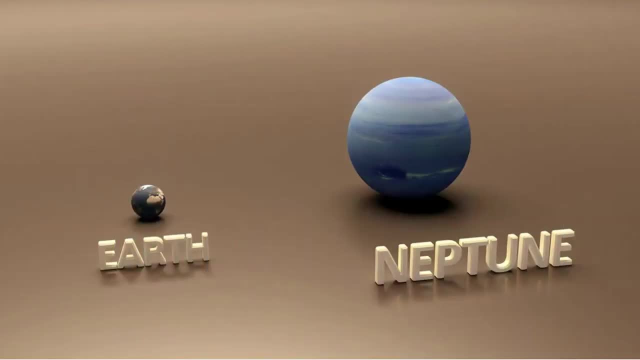 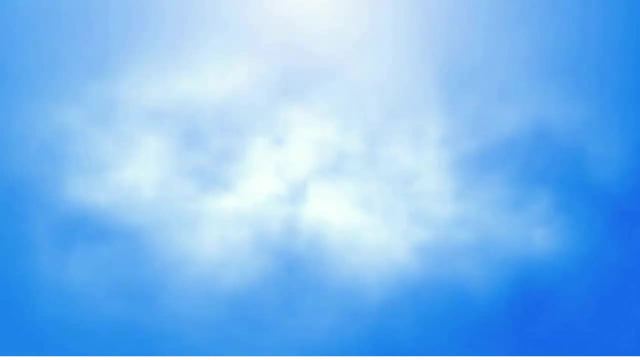 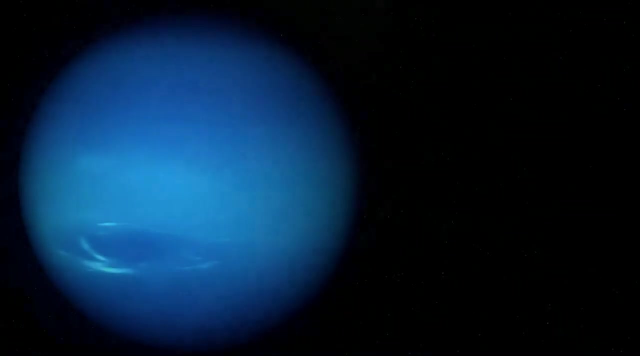 Neptune is four times the size of the Earth. Its surface is mainly a dense, soupy mixture of water, methane and some ammonia. It is made up of methane and ammonia that surrounds a small dense, solid core. Its atmosphere is mainly hydrogen helium and around 1% methane. 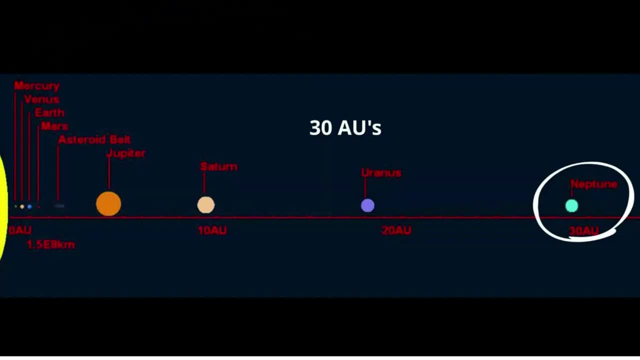 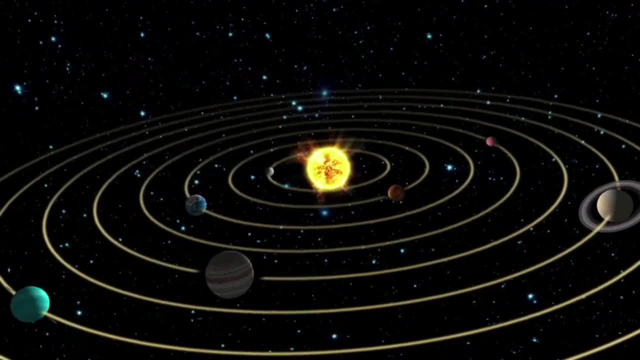 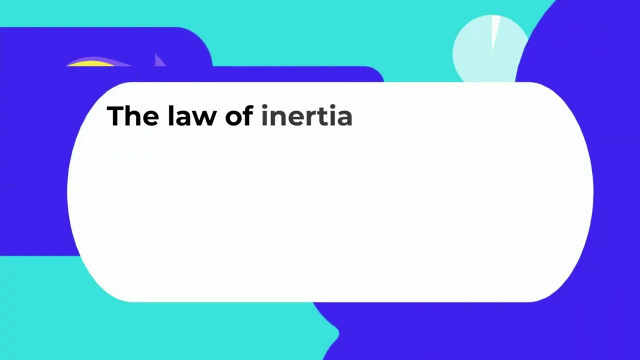 Neptune is 30 AUs from the sun and no life has been detected on Neptune. Planets revolve around the sun because of two forces are at work: inertia and gravity. The law of inertia says that an object in motion will tend to stay in straight-line motion. 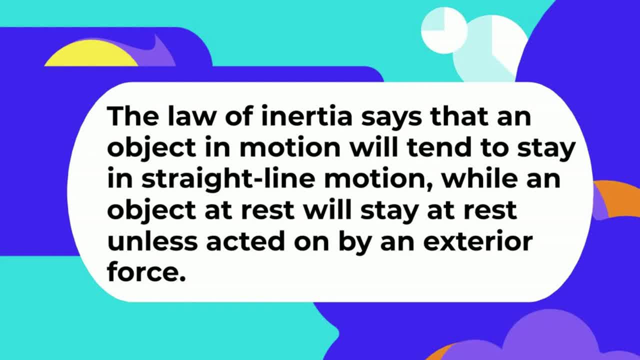 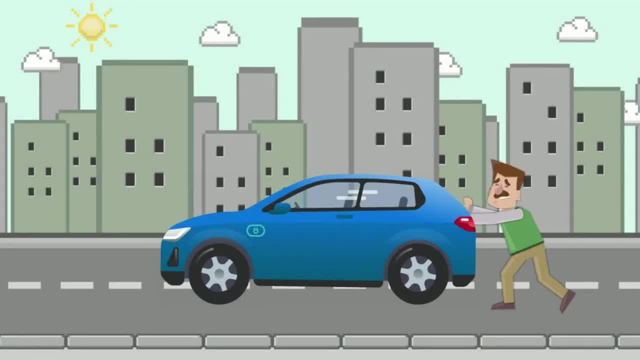 while an object at rest will stay at rest unless acted on by an exterior force. For example, if you have tried to push a heavy object like a car, you know that it is hard to get it moving. This is because it will tend to stay at rest. 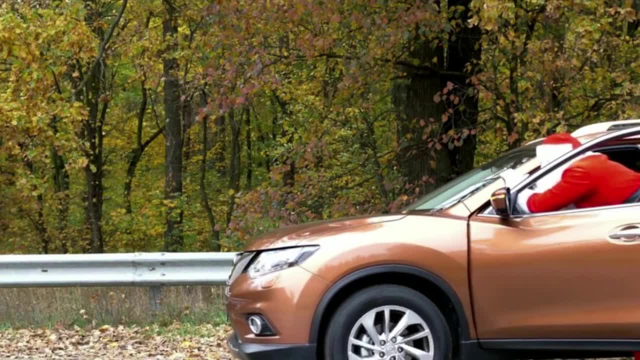 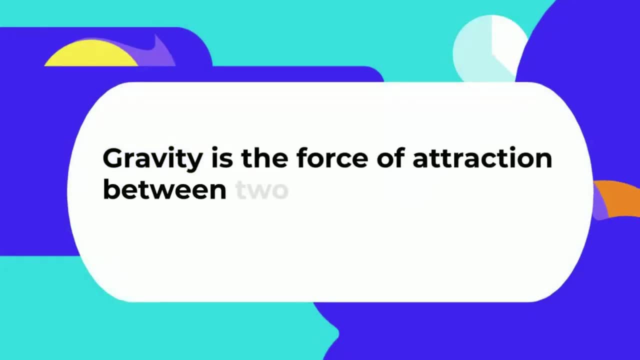 But once it starts moving it becomes a little easier, as inertia tends to keep it moving. Gravity is the force of attraction between two objects. It is a fundamental force in the universe that causes every object to be attracted to every other object. When you jump upward, you can feel the force of gravity pulling you back to Earth. 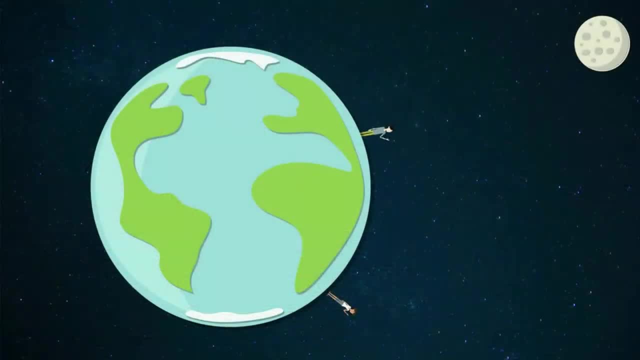 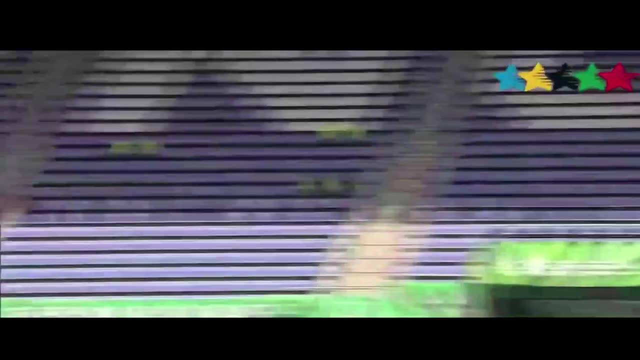 The greater the mass of an object, the greater the force of gravity. As this hammer-thrower spins, we know when he releases the ball it will travel in a straight line, But the handle, and him holding onto the handle, acts like gravity. 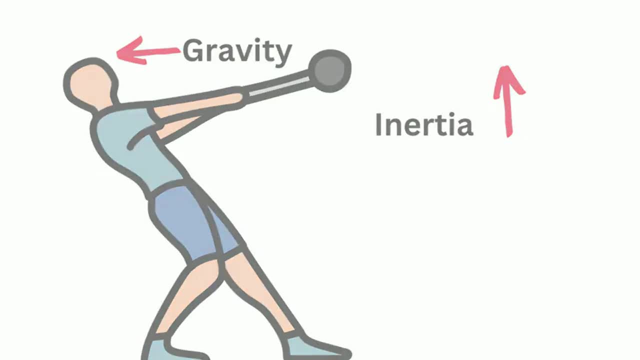 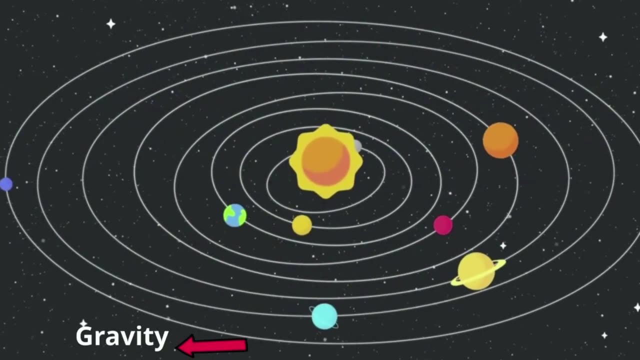 and keeps the hammer spinning in a circle. In a similar fashion, gravity and inertia work together to keep the planets in orbit. Gravitational force is pulling the planet inward and the planet's inertia is trying to make it move in a straight line. 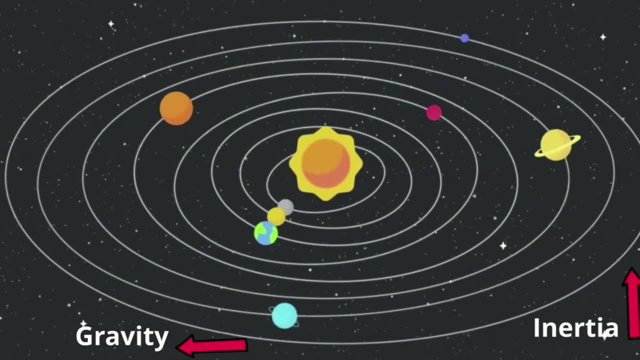 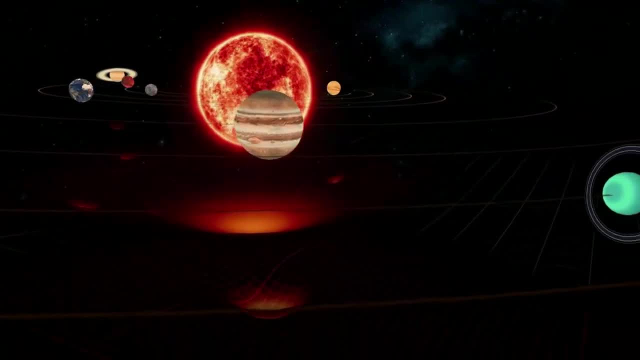 This creates a circular or elliptical orbit around the Sun. Again, the planet's inertia causes it to move forward in a straight line, while the gravitational force continually bends its path towards the Sun. As a result, the planet stays in an orbit. 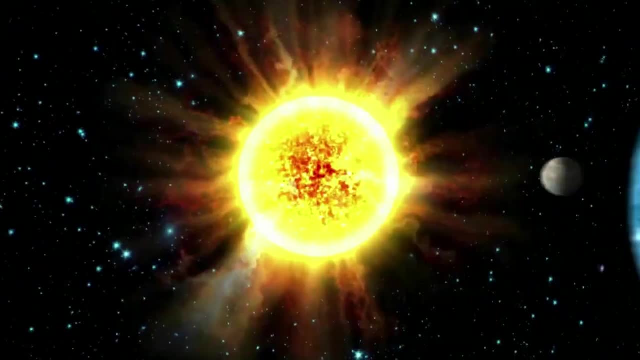 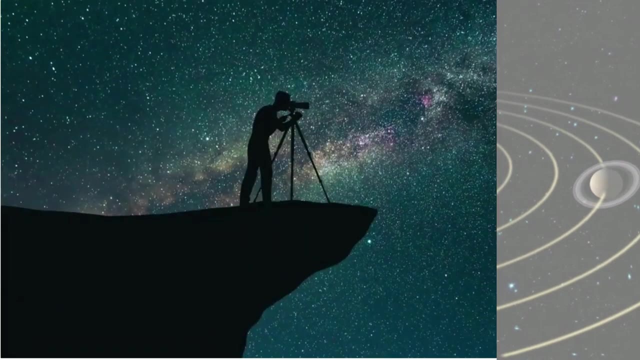 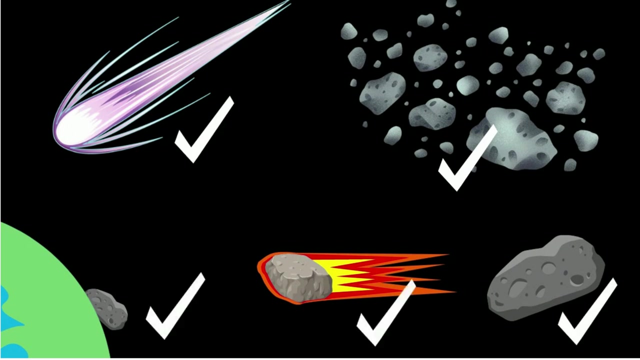 It is a combination of falling towards the Sun due to gravity, but never reaching it due to its forward motion of inertia. In this video, let's learn the difference between an asteroid, comet, meteoroid, meteor and meteorite. An asteroid is an object that is neither a true planet nor a comet that orbits the Sun. 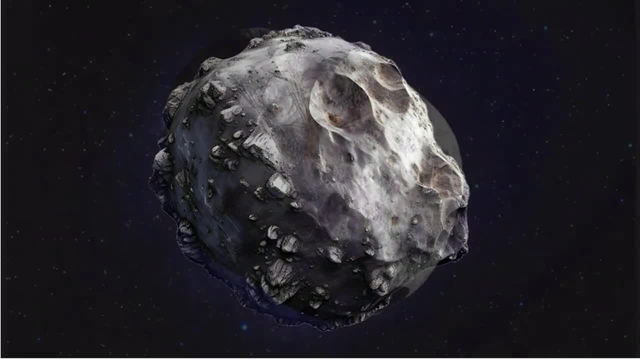 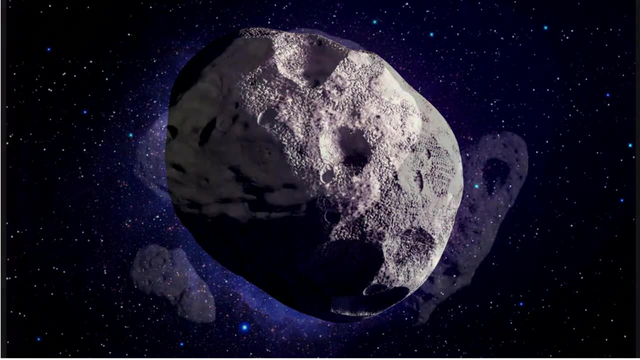 As a result, they are considered minor planets. They are rocky, metallic, or I say bodies with no atmosphere. Sizes and shapes of asteroids vary greatly, ranging from one meter rocks to almost a thousand kilometers in diameter, The greatest number of asteroids. 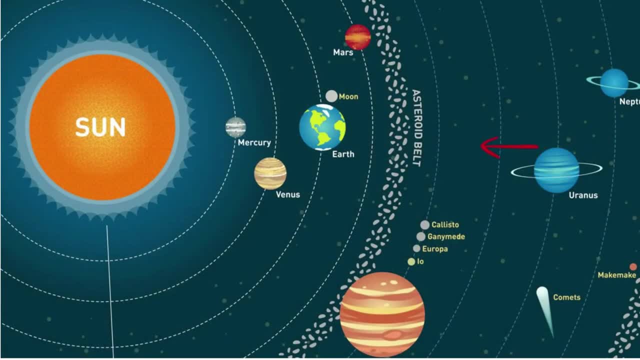 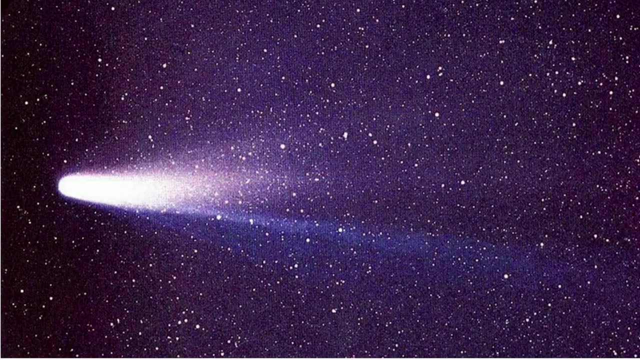 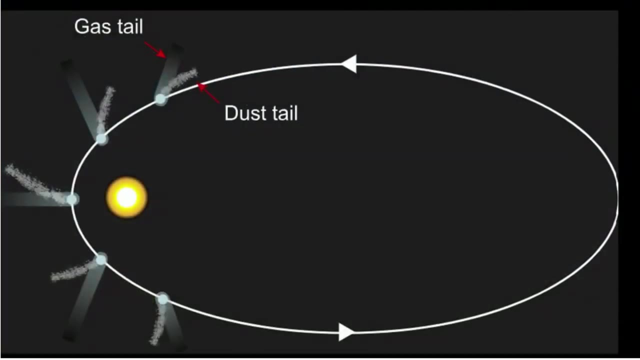 are located between the orbits of Mars and Jupiter in the main asteroid belt. A comet is an object made of frozen ice, gas and dust that orbits the Sun. They are classified as a small solar system body. Many comets have a very elliptical. 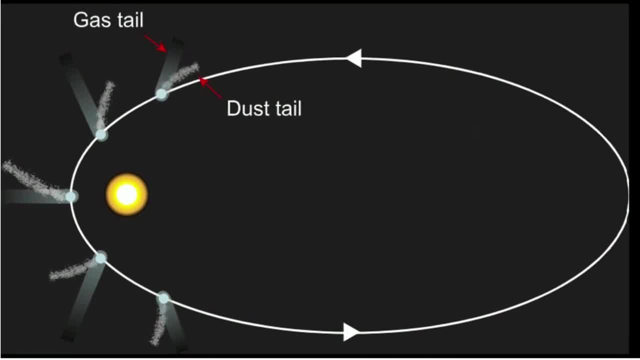 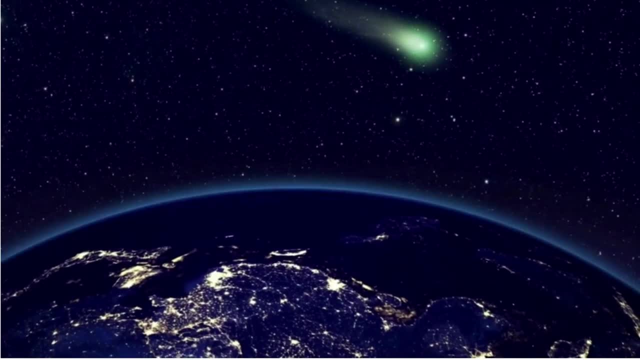 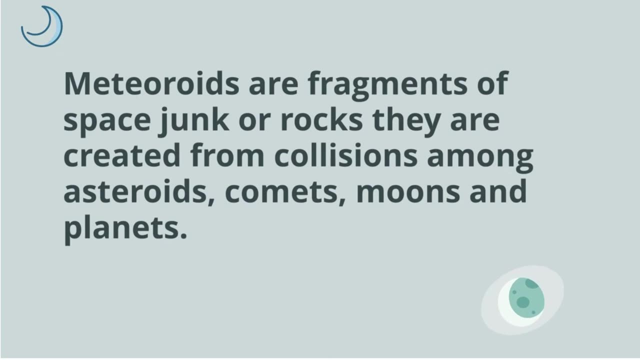 orbit and, as the comet gets closer to the Sun, heats up and forms a glowing tail. As of 2021, there are 4,584 identified comets and roughly one comet is visible without a telescope. a year. A meteoroid? 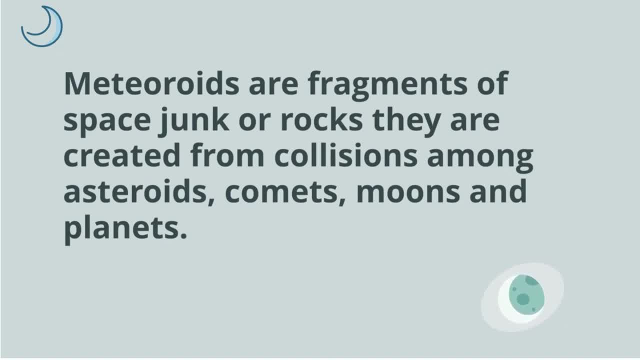 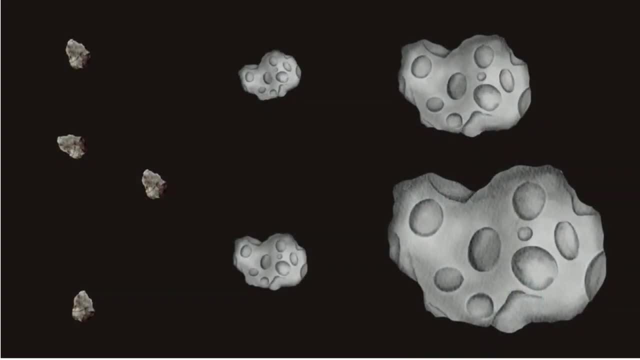 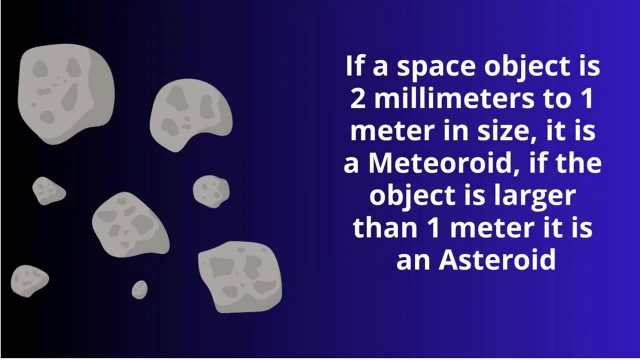 are fragments of space junk or rocks that are created from collisions among asteroids, comets, moons and even planets. Meteoroids are smaller than asteroids, ranging in size from grains of rock to ice to objects up to a meter wide. They are among the. 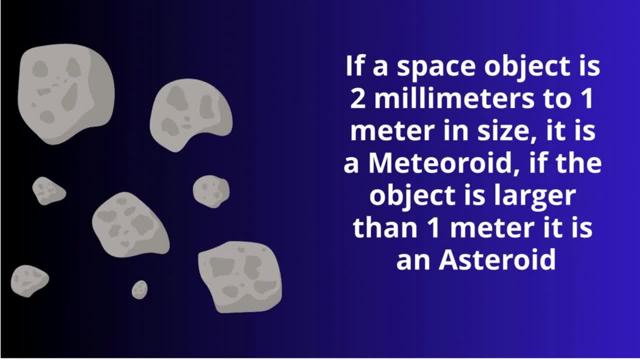 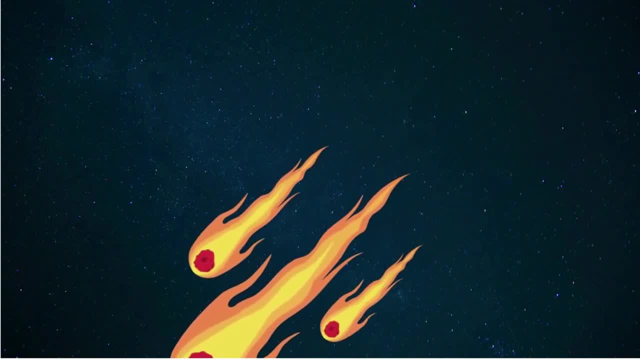 smallest space rocks that orbit the Sun. A meteor is a meteoroid that passes through the Earth's atmosphere. It then heats up due to air resistance and glows brightly. In this clip, you can see some of the meteors flash by. 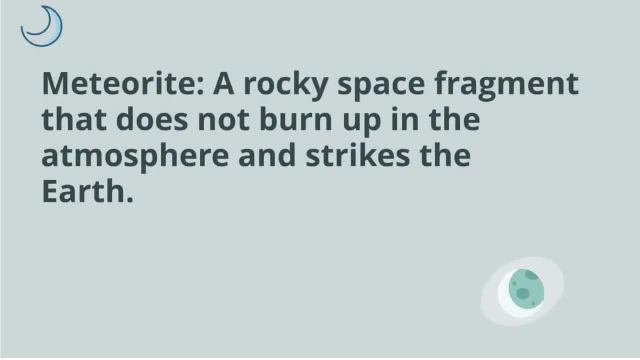 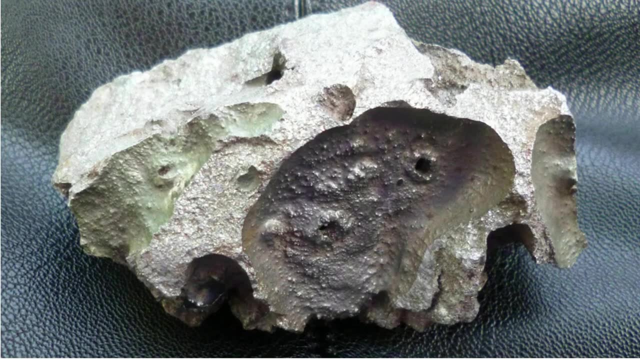 A space fragment that does not burn into the atmosphere and strikes the Earth is called a meteorite. Here are some pictures of actual meteorites that struck the Earth. Now here's the sequence: You have a meteoroid in space and when it enters, 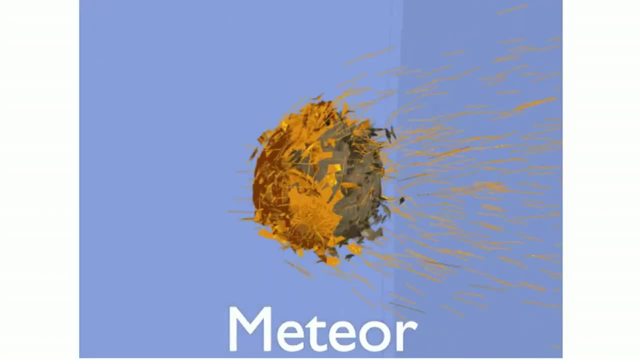 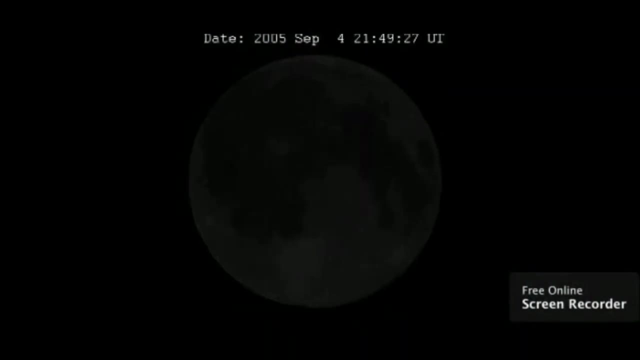 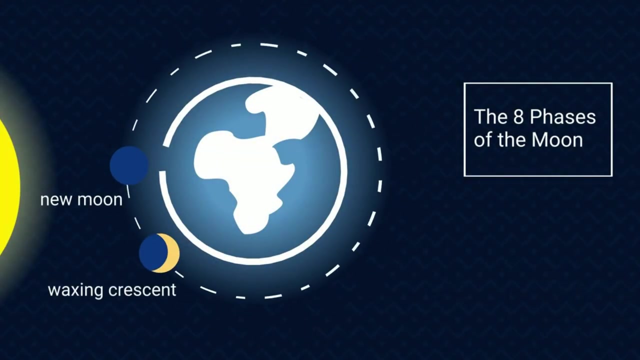 the atmosphere, it is a meteor, and when it strikes the Earth, it is a meteorite. As the Moon revolves around the Earth, its appearance changes and cycles through eight different phases. The eight phases are: New Moon- Waxing Crescent. First Quarter Waxing Gibbous. 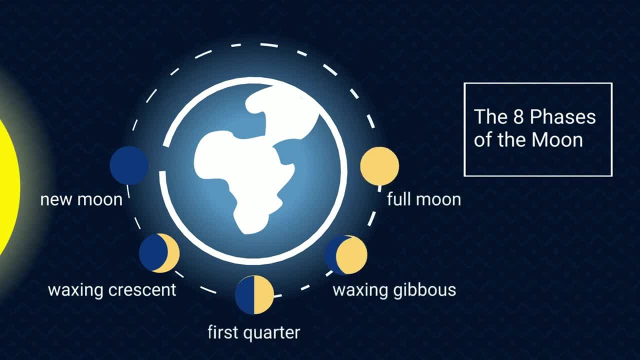 Full Moon, Waning Gibbous, Third Quarter, Waning Crescent, and then you're back at New Moon. So let's get to work on learning these phases. First, the Moon revolves around the Earth in a counterclockwise direction. 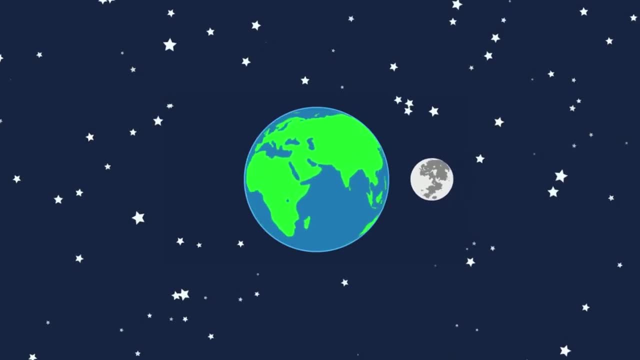 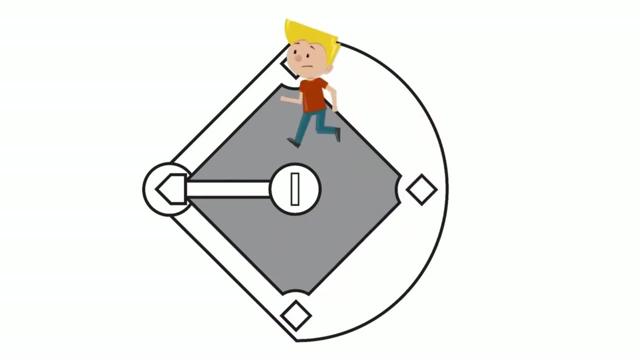 An easy way to remember counterclockwise is to think about running the bases during a baseball game. You run in a counterclockwise direction. So let's begin at New Moon, which would be Home Plate. It occurs when the Moon is between: 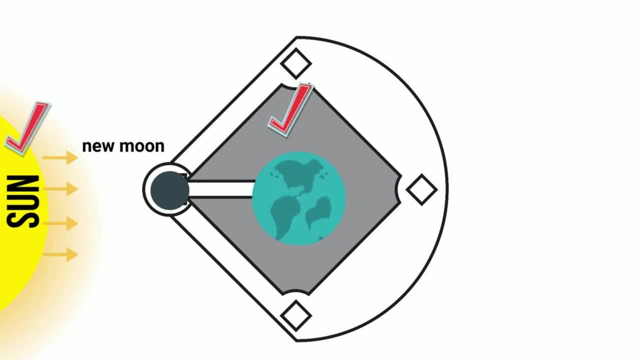 the Earth and the Sun. First base would be First Quarter. Second base would be Full Moon, which occurs when the Moon is beyond the Earth and reflects the sunlight back. Third base is Third Quarter and then you're back at New Moon When you move from. 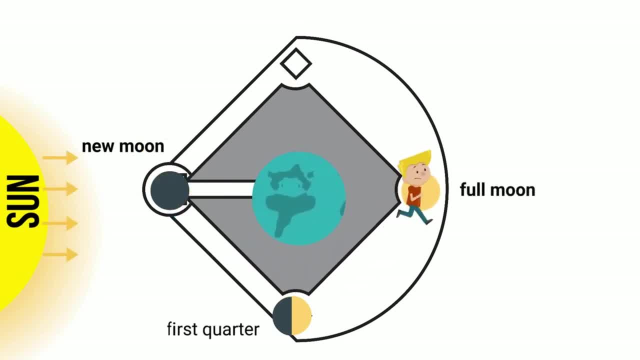 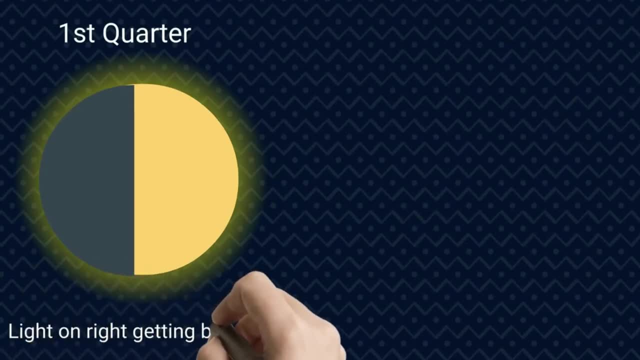 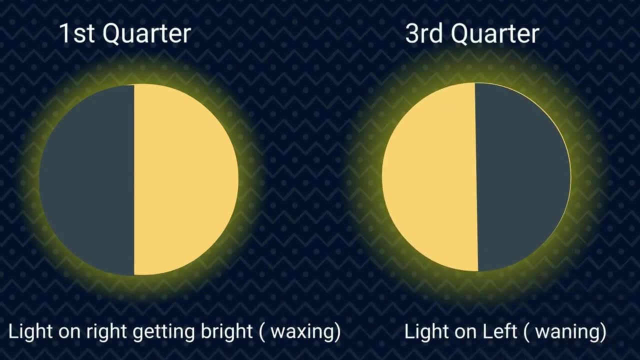 New Moon to Full Moon, the light is growing, which is called Waxing. An easy way to remember this is with the saying Light on Right Getting Bright, which is Waxing. The light is waning When you go from New Moon. 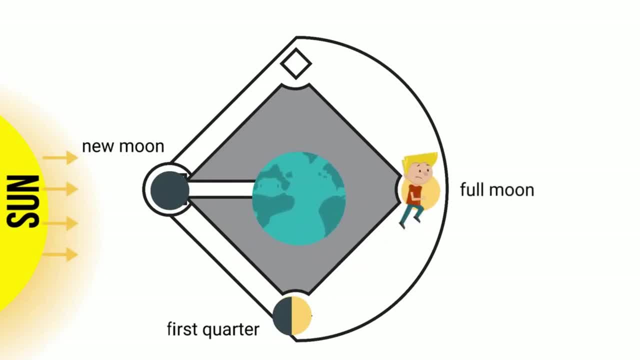 to Full Moon, the light is on the right, so you are waxing and the light grows. When you go from Full Moon to New Moon, the light is on the left. you are waning and you are subtracting light. 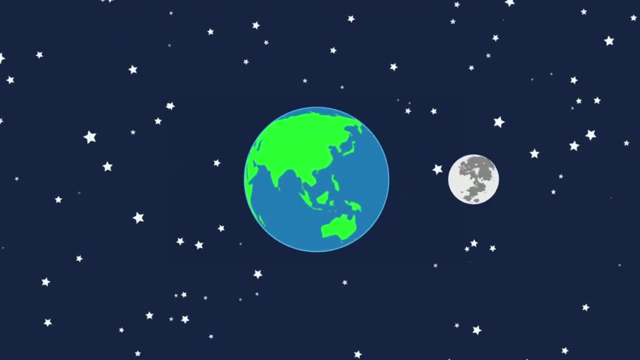 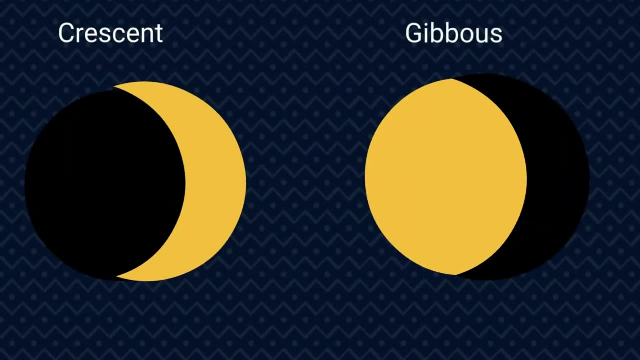 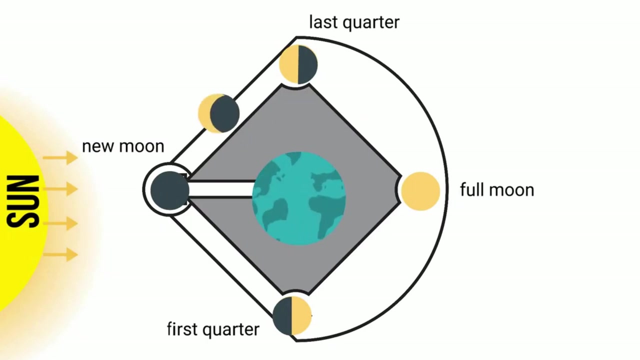 Now you have two more moons to think about: Crescent and Gibbous. A Crescent Moon has a small amount of light, whereas a Gibbous Moon has a great deal of light. An easy way to remember where these are located is that a Crescent Moon. 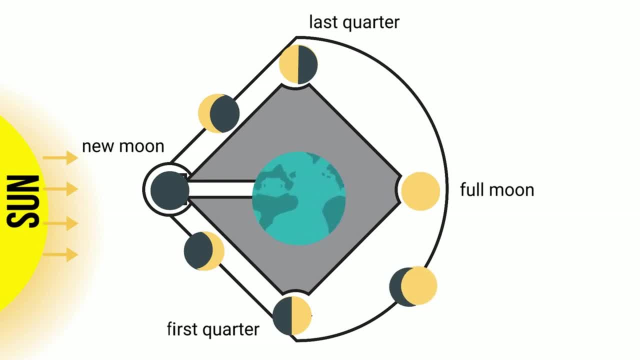 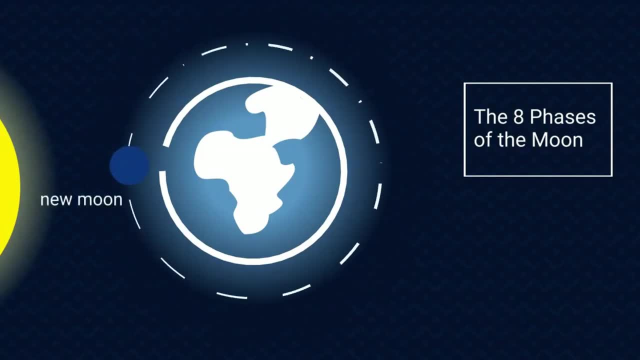 always appears before and after a New Moon, and a Gibbous Moon always appears before and after a Full Moon. So now let's put this together. You have New Moon. light is on the right third quarter, then a waxing Gibbous. 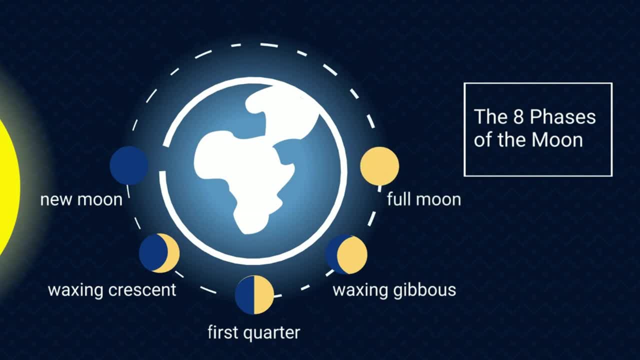 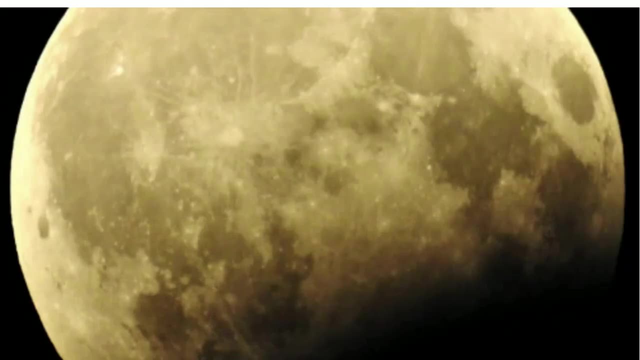 now you are at Full Moon. now you go to waning Gibbous and the light now is on the left of the shadow, third quarter, waning Crescent, and then you are back at New Moon. I hope that helps When the shadow of one celestial body 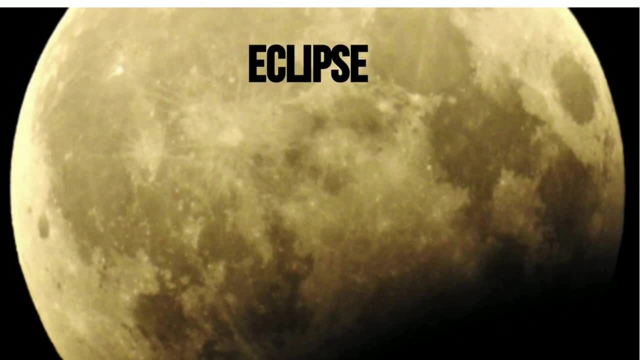 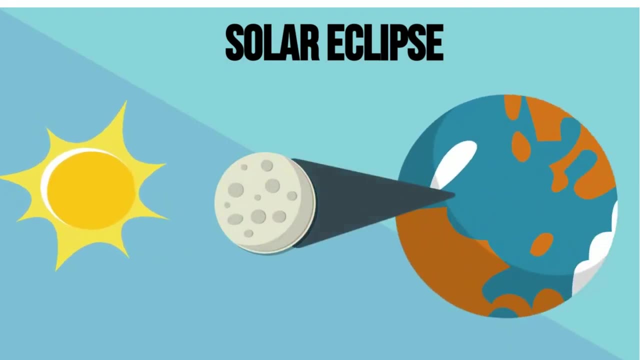 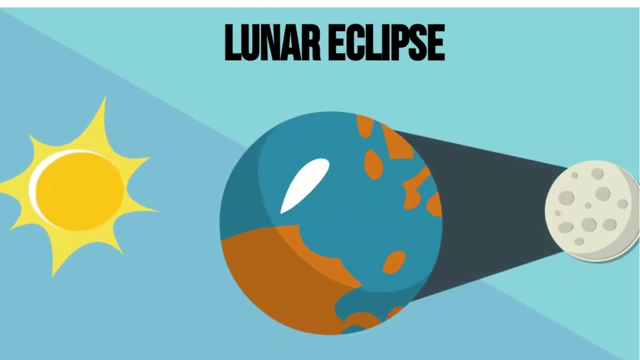 like the Moon or the Earth falls on another, an eclipse occurs. A lunar eclipse happens when the Earth comes between the Earth and the Sun and the shadow of the Moon falls on part of the Earth. A lunar eclipse happens when the Earth comes between 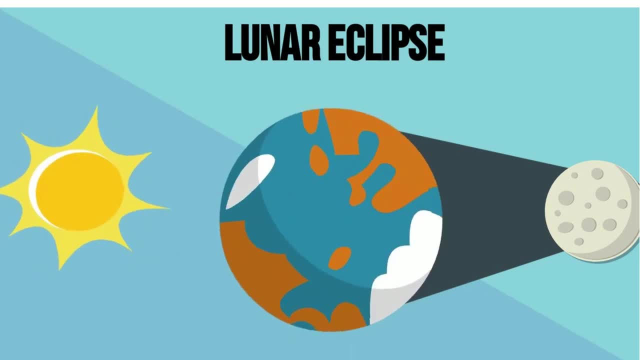 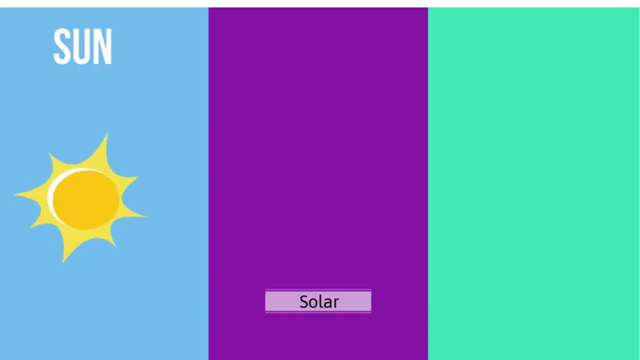 the Sun and the Moon, and the shadow of Earth falls on the Moon. Let's talk about a couple ways to help you remember the difference between a solar and lunar eclipse. The order of the celestial bodies during a solar eclipse is Sun, Earth. 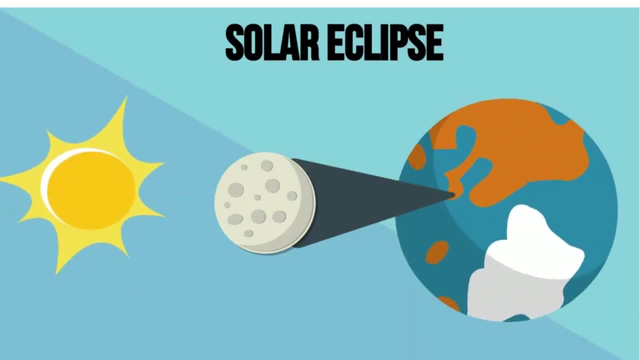 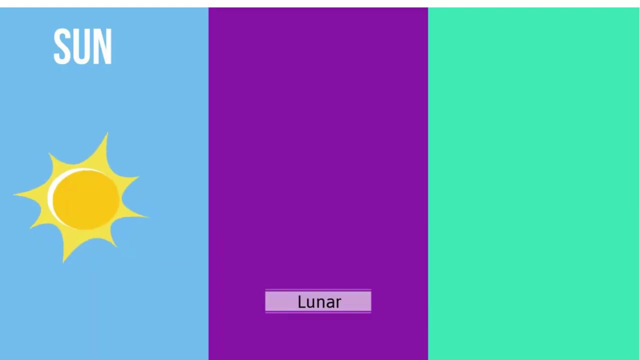 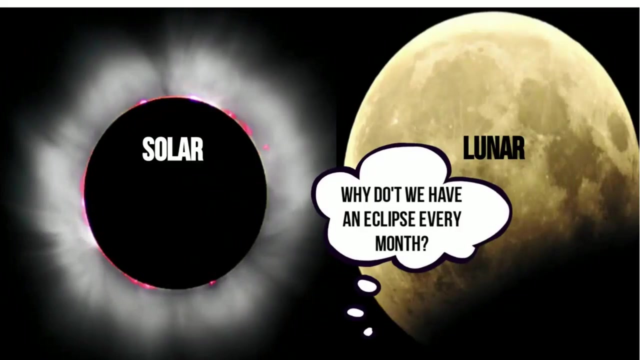 Moon or Sim. Next, you may be wondering why you don't see a solar and lunar eclipse. during a lunar eclipse, The order of the celestial bodies is Sun, Earth, Moon or Sim. Why you don't see a solar and lunar eclipse. 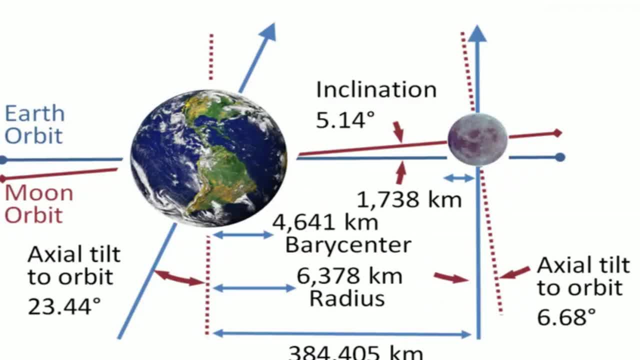 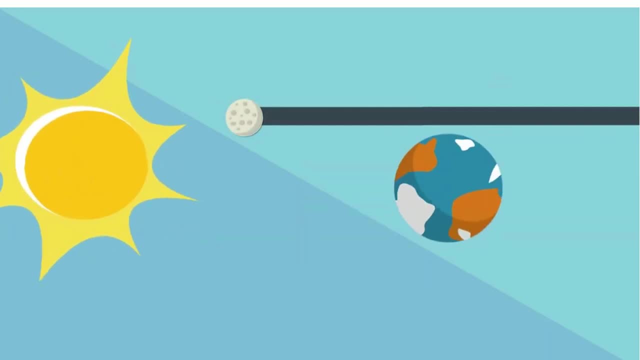 every month. The reason is that the Moon's orbit around the Earth is tilted by about 5 degrees relative to the orbit of the Earth around the Sun. This tilt is just enough to place the Moon out of the Earth's shadow for most full moons. 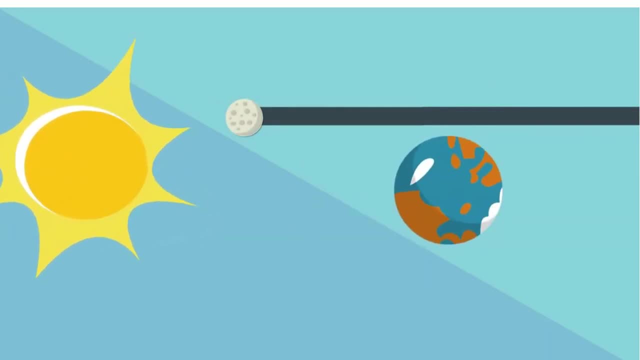 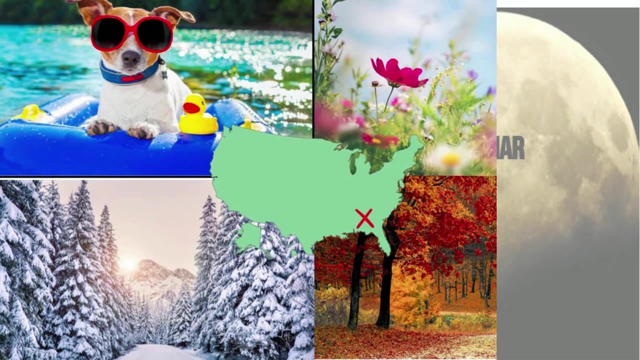 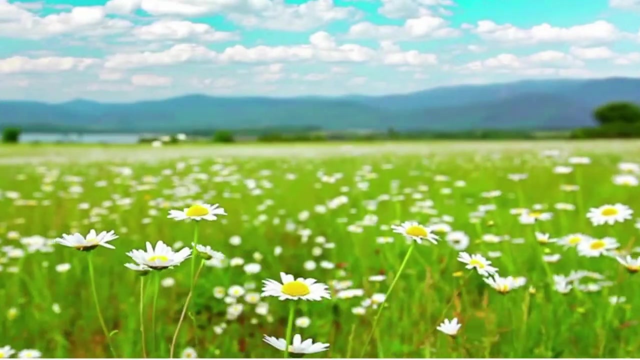 and the Earth out of the Moon's shadow for most new moons. So there we go, two different types of eclipses, a lunar eclipse. I live in the southern portion of the US and therefore have the joy of experiencing seasons. I really enjoy summer. 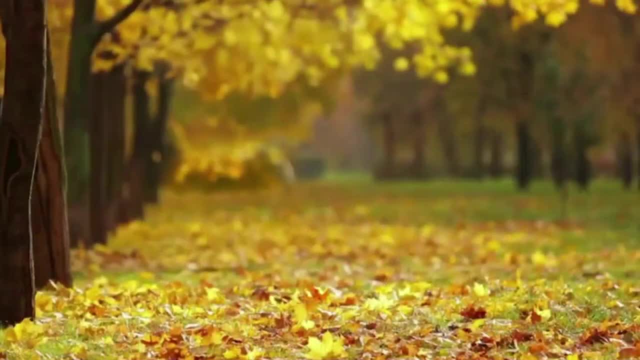 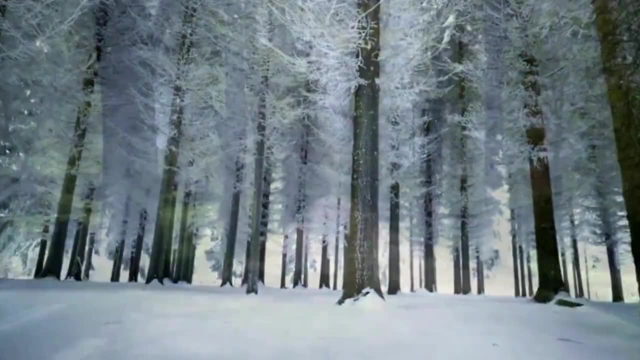 but then after a while I look forward to fall and cooler temperatures. Once I get used to cold temperatures, I appreciate the winter, But near the end I can't wait for spring to arrive. In reality, seasons only occur in two regions of the world. 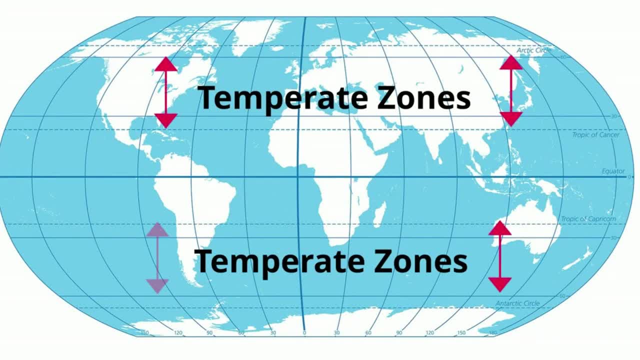 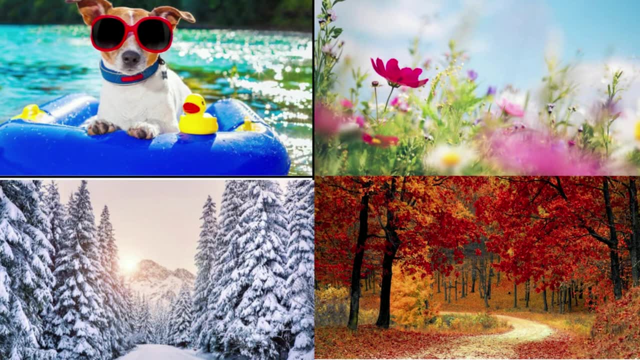 They are the temperate zones 23.5 degrees north and south and 66.5 degrees north and south. In the northern hemisphere spring begins around March 21st, summer around June 21st, autumn around September 23rd. 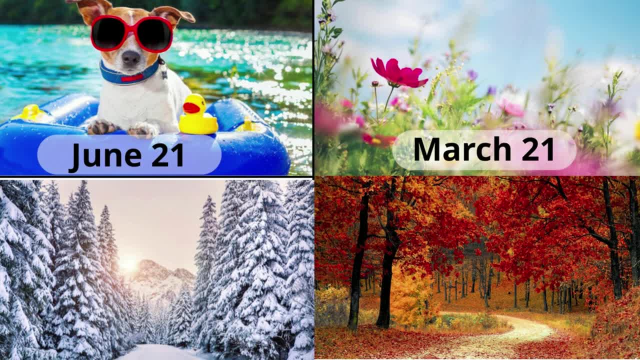 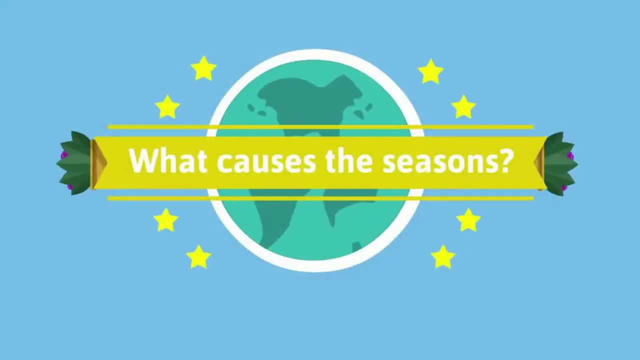 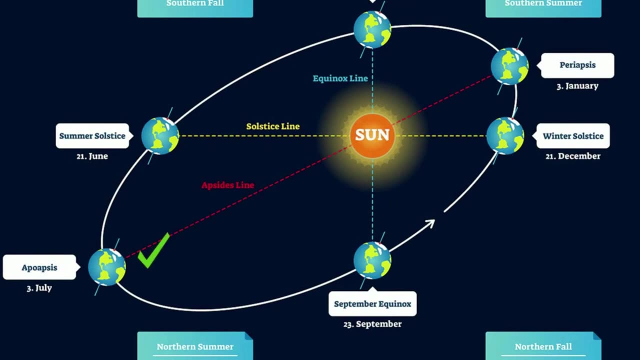 and winter around December 21st. But what causes the seasons? It would make sense that the winter occurs when the Earth is furthest from the Sun and summer occurs when the Earth is closest to the Sun, But in reality it is almost the opposite. 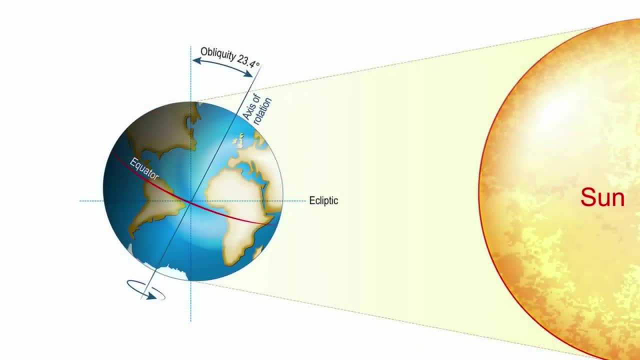 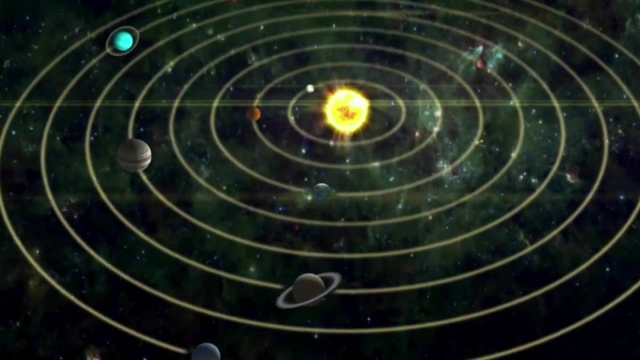 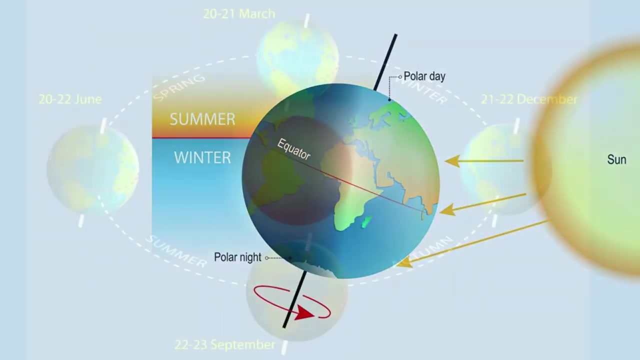 The main reason for seasons is that the Earth is tilted on its axis. The Earth sits at 23.44 degrees As the Earth revolves around the Sun. this tilt of the Earth's axis causes sunlight to strike certain regions of the Earth at different angles. 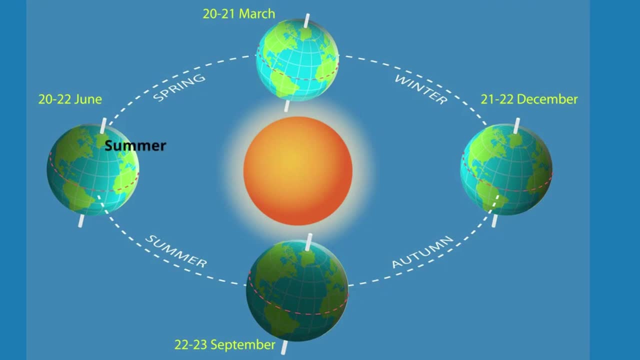 The hemisphere that is tilted towards the Sun is warmer because sunlight travels more directly to the Earth's surface and, as a result, there is more energy per square kilometer. Winter occurs when the hemisphere is pointed away from the Sun. This results in the sunlight striking 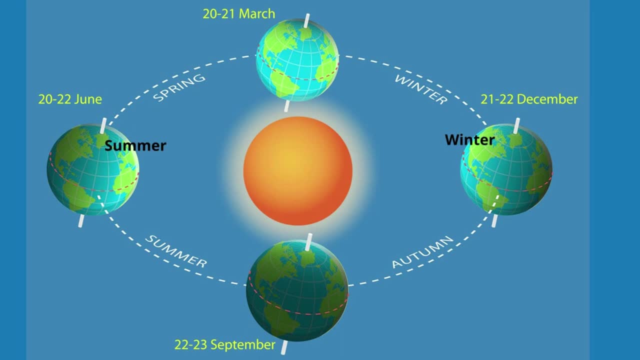 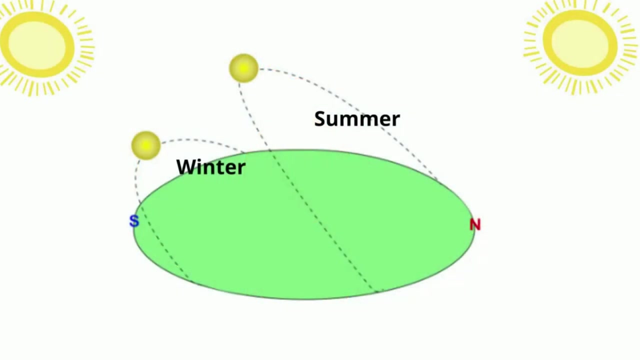 the Earth at a more indirect angle, and this results in less energy per square kilometer. During spring and fall, the angle of the Sun is in between the winter and summer, and that is why the temperature is somewhere between summer and winter. This also causes the hemisphere.